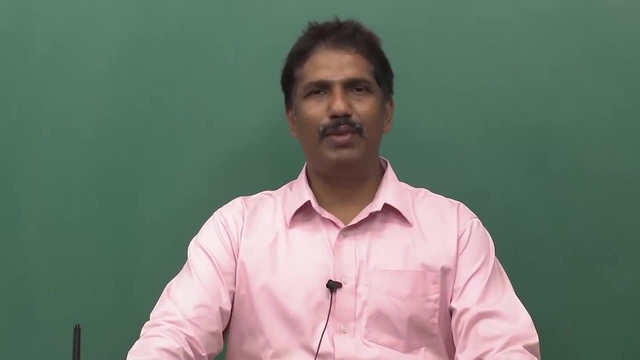 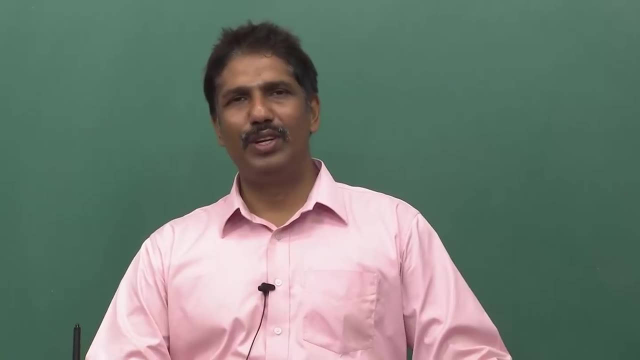 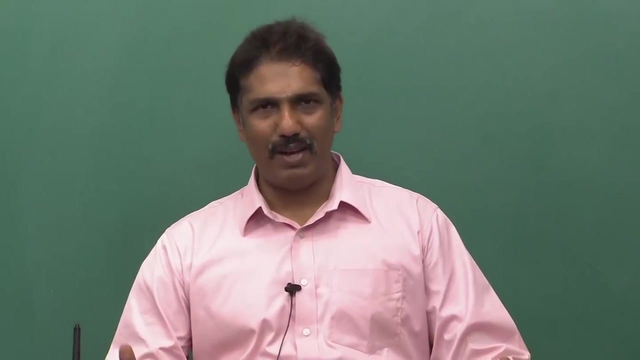 customer demands. So that is why today you see many products which are in the market. talk about smart phones, intelligent phones, smart material, intelligent material. So many new things come. All these things are getting inspired from nature. So composites are manmade and now we are moving towards bio-mimicking composites. We will try to see. 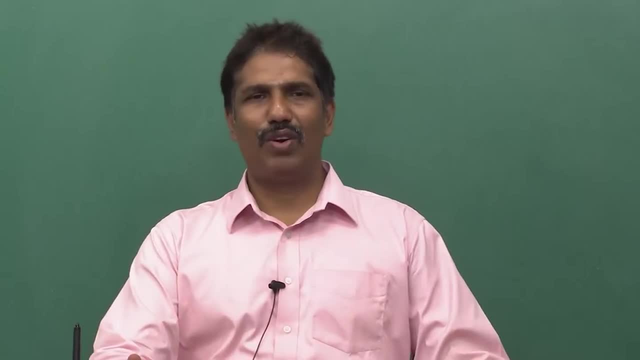 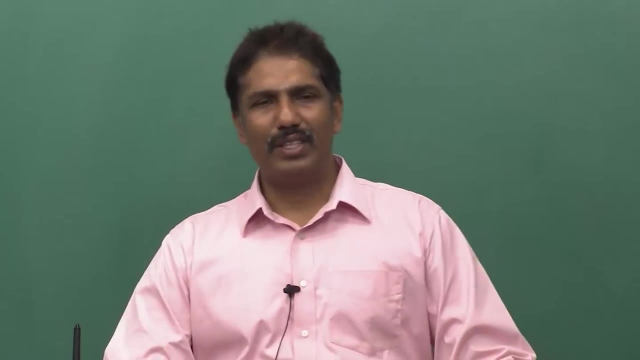 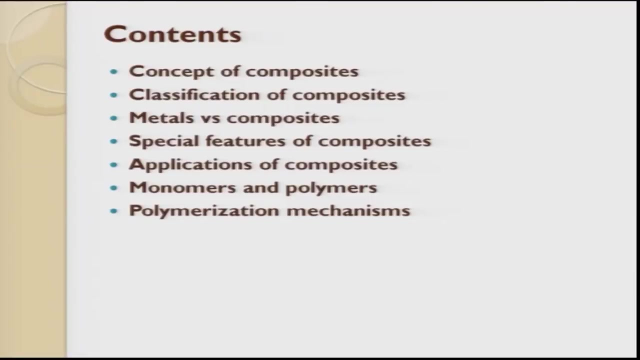 some of the bio-mimicking composites in the last phase of this course. So in today's lecture what we are trying to cover is we will try to cover the content of composites, then we will talk about classifications of composites. then what is the advantage? 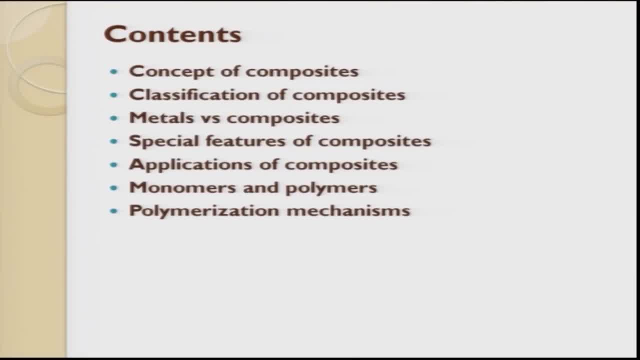 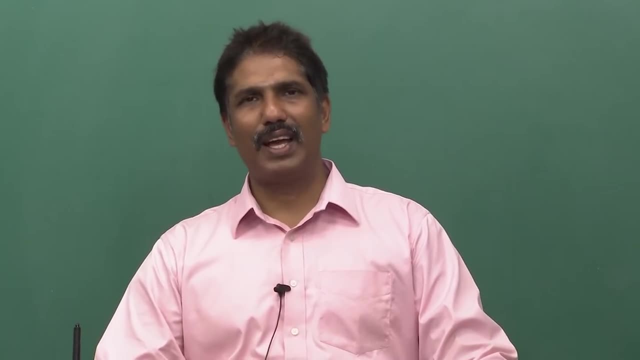 of composites as compared to that of metals. We will talk about different features of composites, applications of composites. then we take exclusively polymer matrix, composite, and we will talk about what is monomer, what is polymer, what are the different, what are the different mechanisms, where, in which this polymerization can happen. 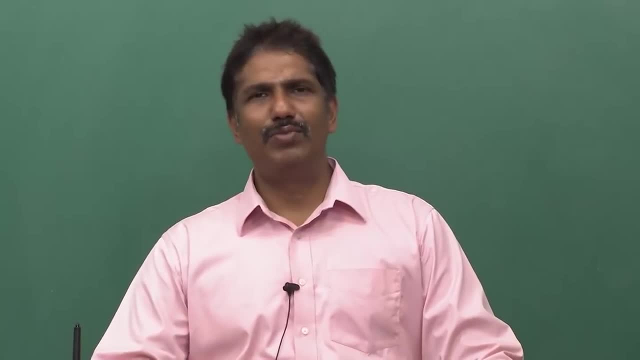 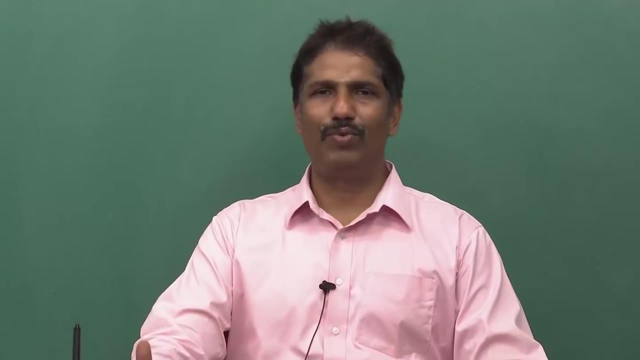 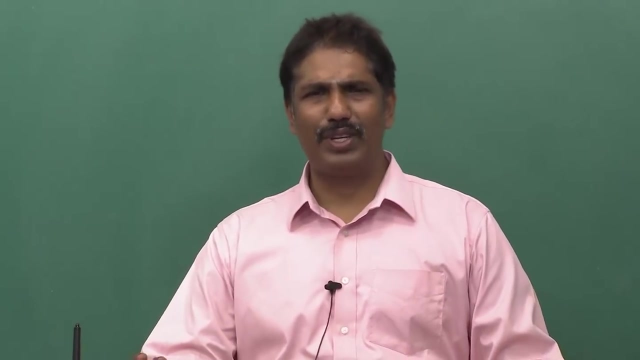 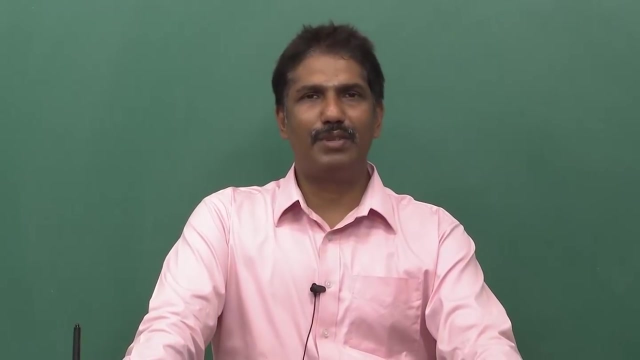 So what is composite? Though composite is a term which is used almost for a century, still a clear definition has not been evolved. So, based on my understanding and with their literature available, I have just put a very broad sense of definition of composites. So, in a broad sense, the term composite materials, 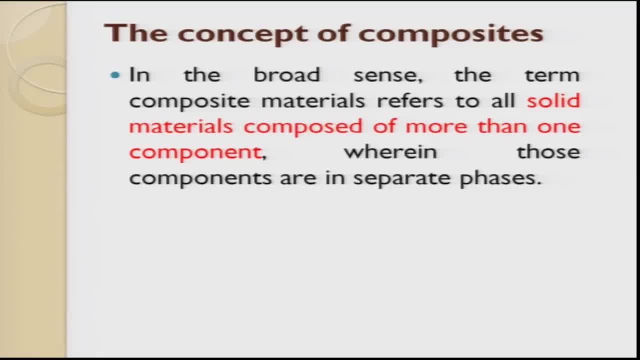 refers to a solid matter composed of more than one component, wherein those components are in separate phases. So, for example, I take material A, I take material B, I when I mix these two underomposites. So you could see that the material A makes papers and for these paper and later small pieces are pulled apart, the mixture insideовые. 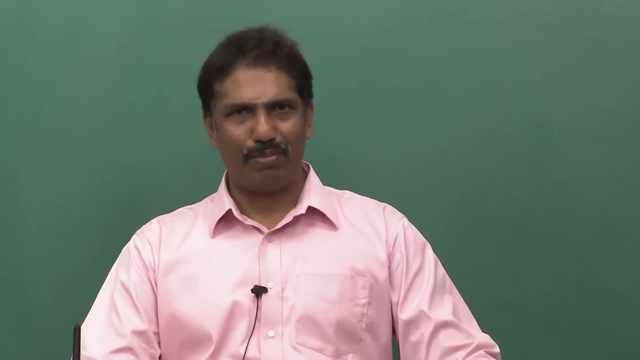 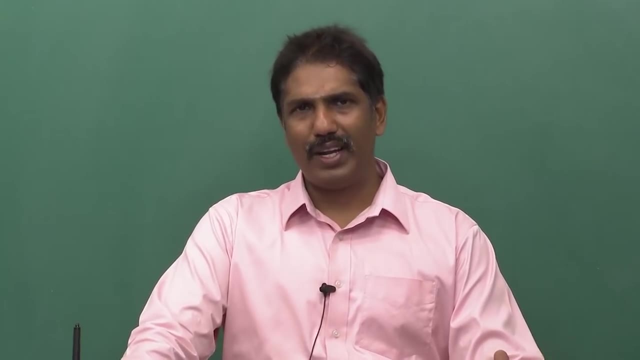 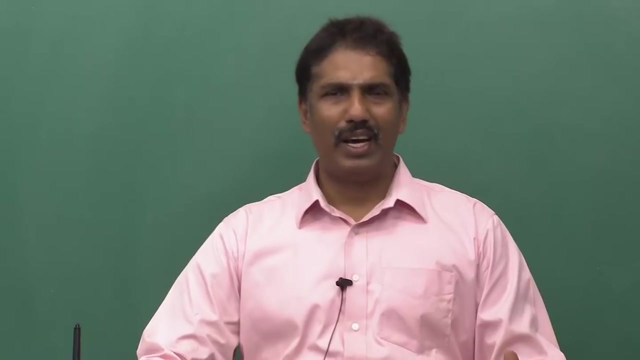 and when I do a process, that means to say I apply pressure temperature with respect to time, then I get a product out. So this product will always be a synergy. so that means to say it will try to take the advantages of A, advantages of B and try to give a new. product where in which that has a required material property. And when I try to take the cross section of the composite material, I can still distinguish what is the component A added, what is component B added. So this is a definition for composites. So the component A is called the matrix and component B is called the reinforcement. So there is a difference between composite and alloy. In an alloy when I try to mix material A plus material B and it forms A product C. the product C which is formed will have a better property, as per the customer's. 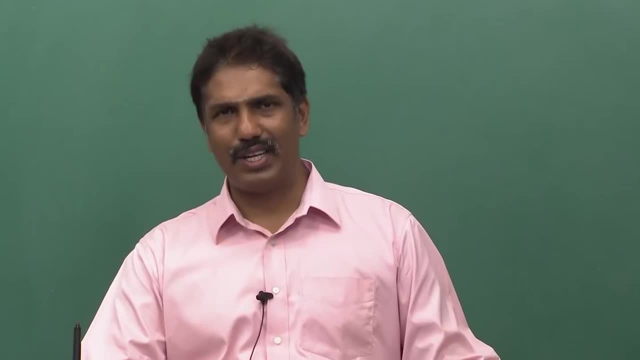 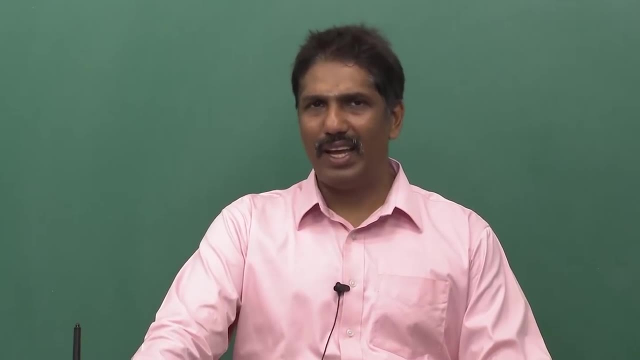 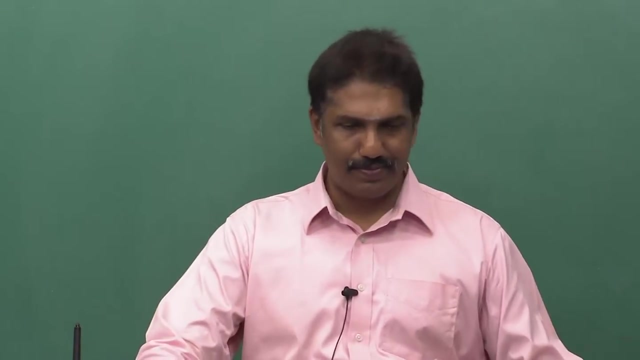 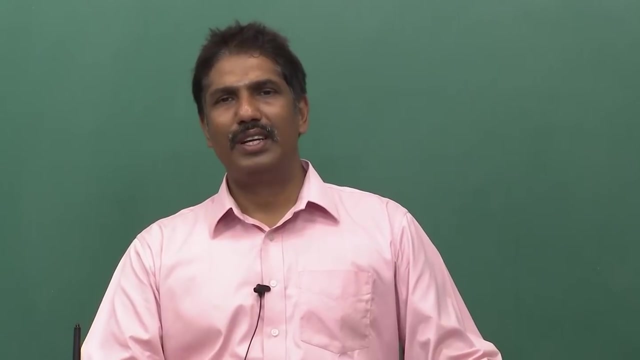 requirement. but when I try to take a cross section, I will not be individually able to detect the presence of material A and B. So this is what is a difference between composite and an alloy. So now let us see the classifications of composite based on the dispersed phase. Here the dispersed phase means the reinforcement. 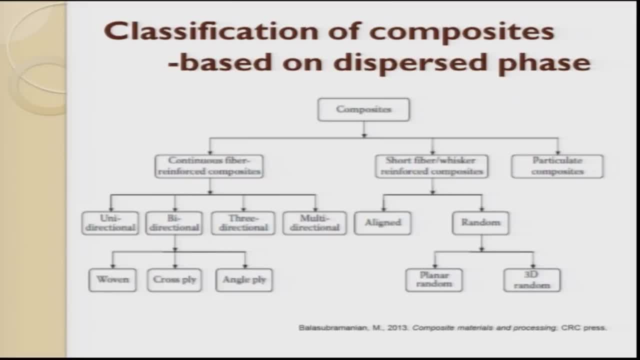 getting dispersed in a matrix. So now it is very clear. you will have two products, which I said: material A, material B, right? So two materials, material A and material B. So material A is called as the matrix, where in which we try to reinforce the component A, and material. 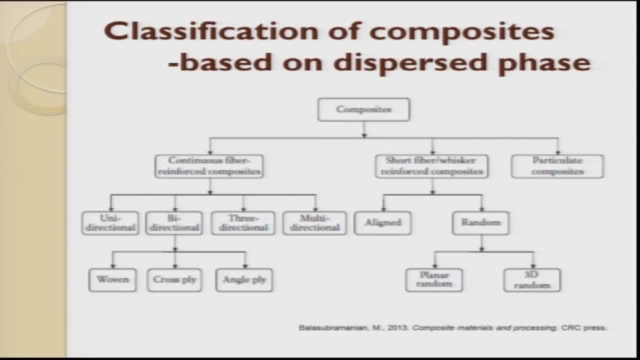 B. So the first classification which is shown here is based on the dispersion of phase. Phase is reinforcement. So here, if you see, composites can be classified into three types. one is called as continuous fiber, reinforced composite, short fiber, reinforced composite, and particulate type- reinforced composites. So long fiber means its length when we talk. 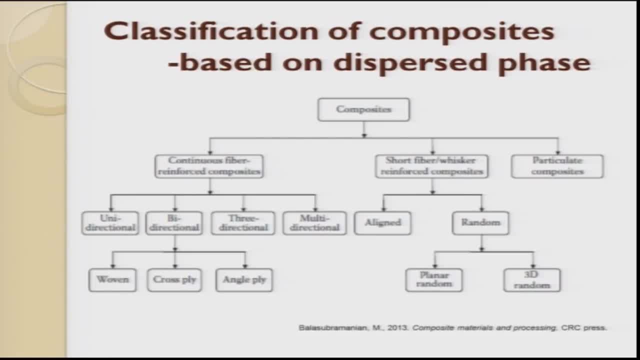 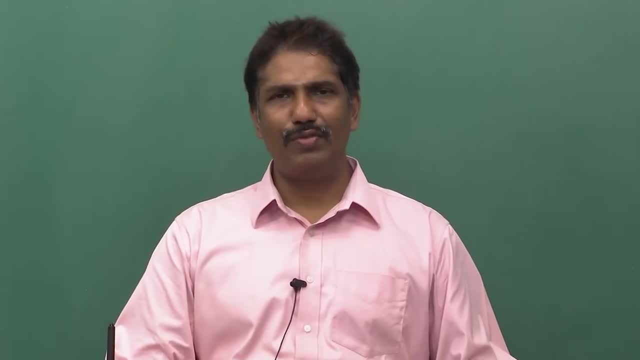 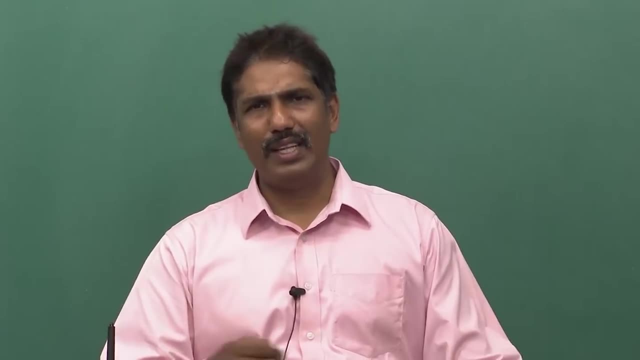 about aspect ratio. If it is length by diameter, we have a long length divided by the diameter of few tens of microns. So these are called as long fibers. It is very similar to that of a thread which is used for stitching the shape and the length right. The next one is short fibers. I cut 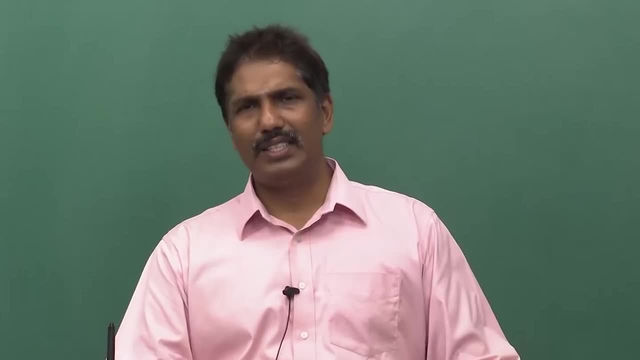 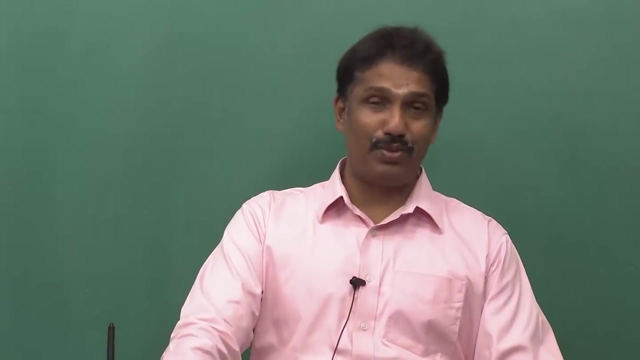 this long fiber into very short fibers and then I try to make something like a mat. So here the aspect ratio is: It is very small. that means to say length is small, diameter will be the same. So these are called as short fibers If the diameter goes very small and if the length is still. 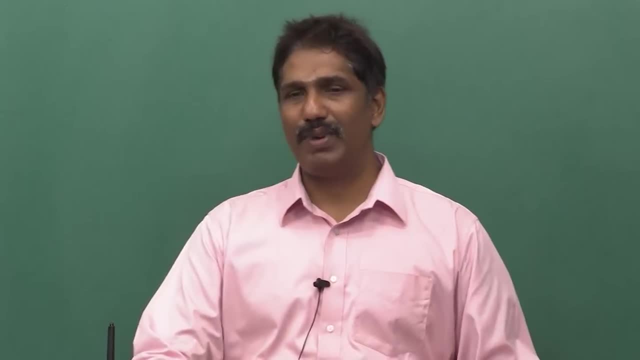 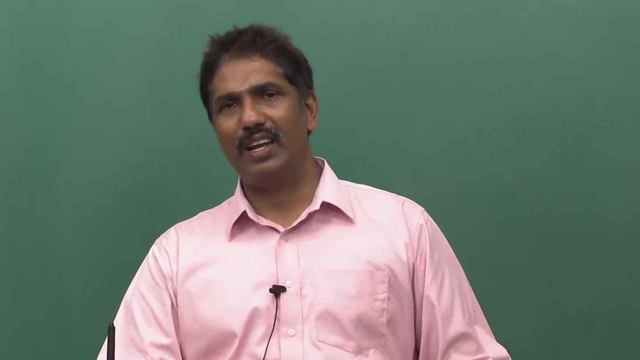 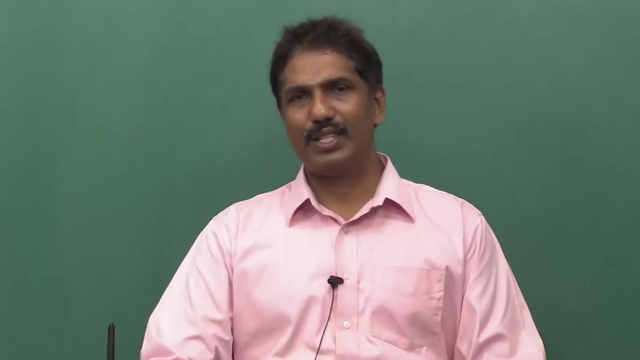 maintained or slightly less. the aspect ratio is maintained. those reinforcement are called as whisker. The difference between short fiber and a whisker is in whisker. the defect densities are very, very low. The third classification here is particulate composites. In particulate composites the reinforcement, whatever we use, will be the 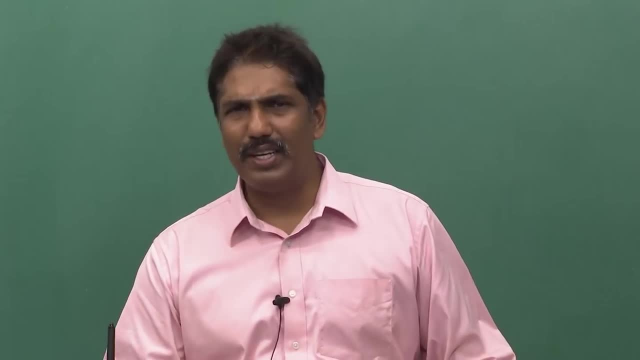 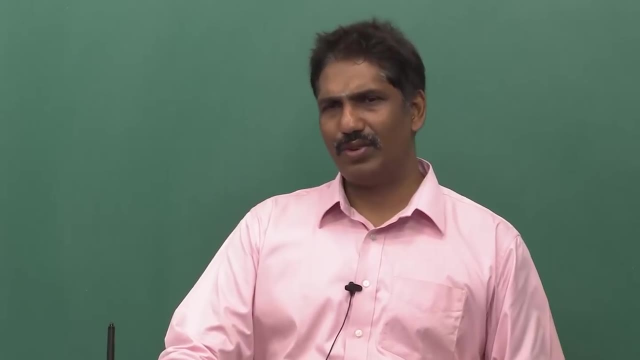 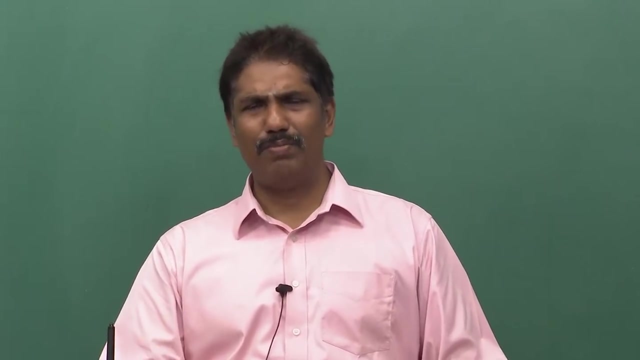 length to diameter ratio will be approximately equal to 1, slightly higher than 1, less than 5, something like that. So it is something like a sand sand size. So those are reinforcing materials. those things are called as particulate composites, So particulate composites are. 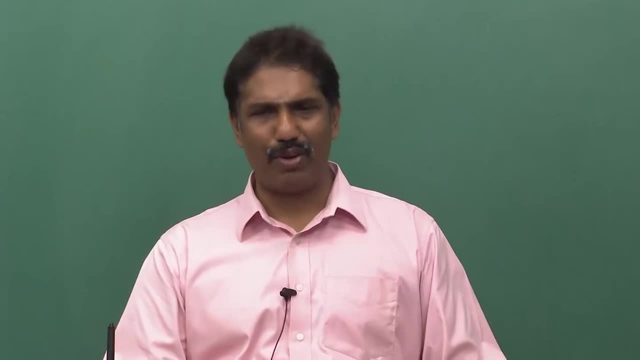 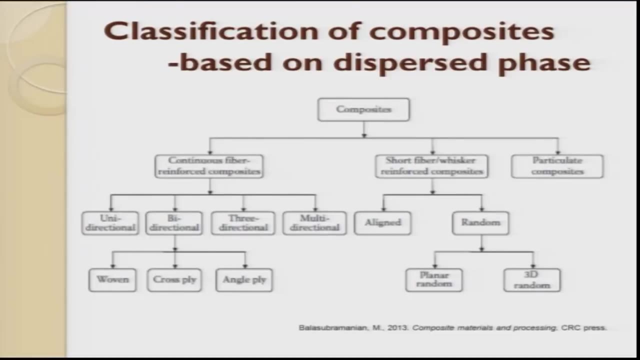 predominantly used in ceramic matrix composite and metal matrix composite. ok, When we go ahead with the continuous fiber reinforced composite, again you have unidirectional, bidirectional. Unidirectional means all the fibers running in one direction length. So bidirection means it is, it is woven like your cloth, your cloth, shirt, what we wear. So you have fibers running. 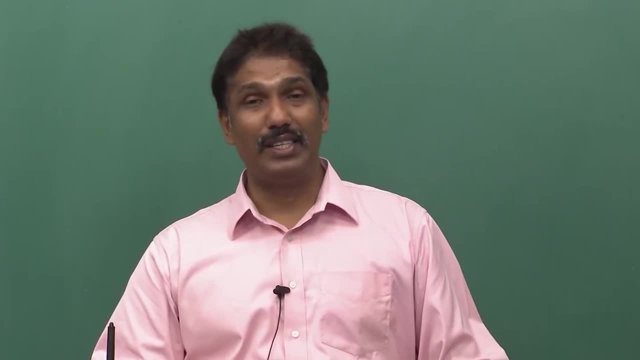 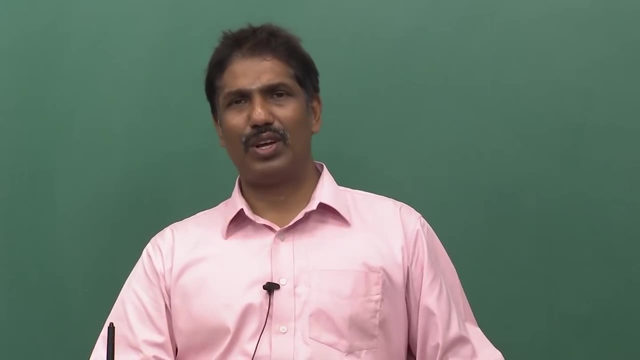 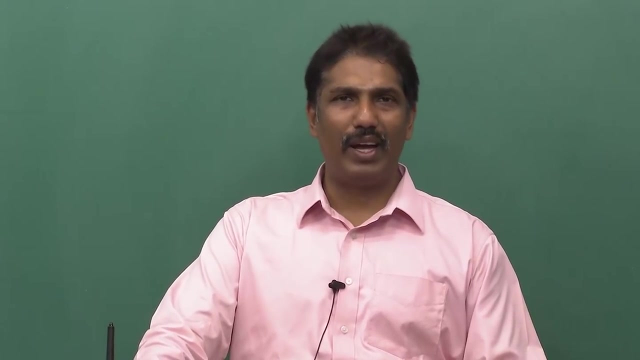 in both direction. You can also have fibers running in the third direction. These composites are now getting into market and it has very high strength and these composites are called as 3D composites, So the fiber runs in all three directions, So that you get x, y and 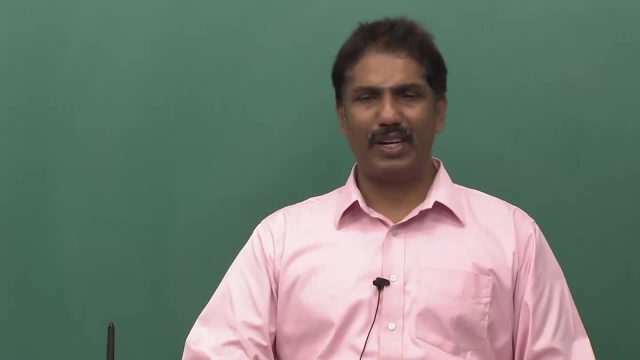 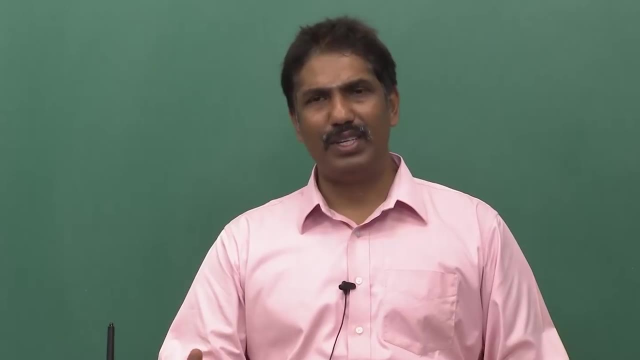 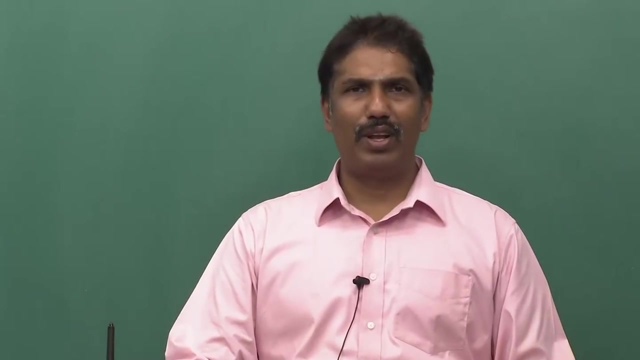 z thickness also. Then you can also have multidirectional. When you talk about short fibers, it can be aligned in one direction or it can be random in nature. So when you go to bidirection we call it as O 1, and then we also call it as there is a classification called as cross. 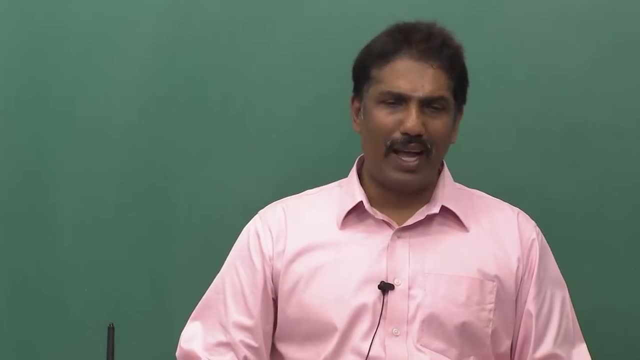 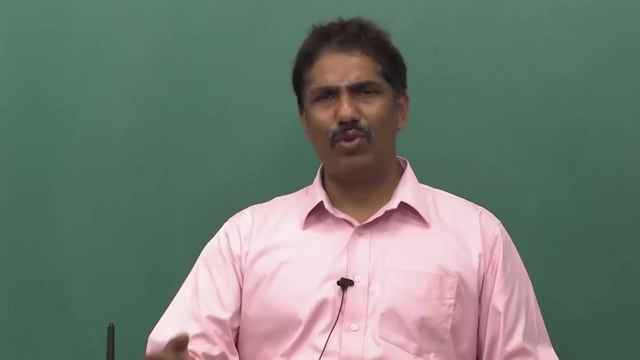 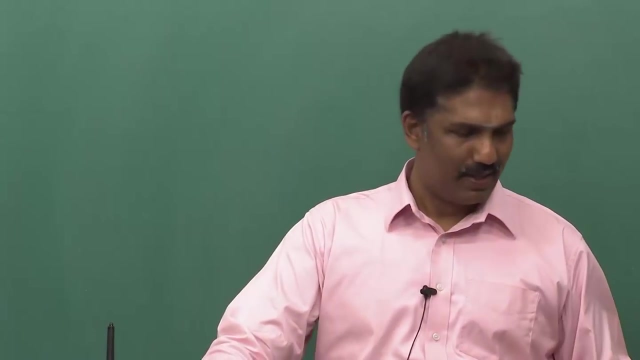 fiber. Then you have angle fibers. So angle fibers- are these textile like material- are cut in different directions and they are laid. So we will see more in detail when we go talk about ah, composite, laminate, laminae and other places, we will see more in details. 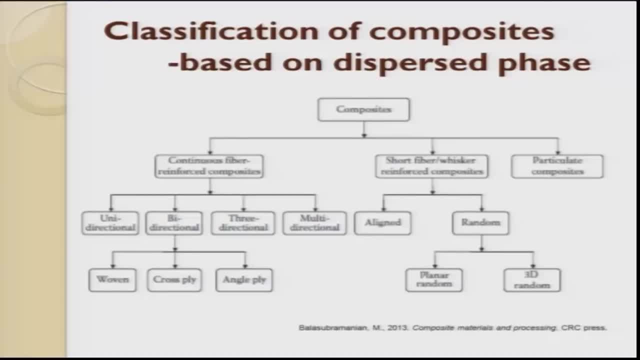 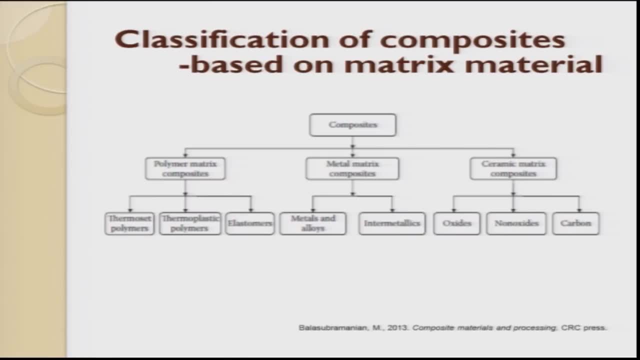 And as far as random is concerned, it can be planar random or it can be 3D random. So when I talk about composites based on matrix classification, there are three types of matrix classification. One is the polymer matrix composite, where this matrix composite is very predominantly. 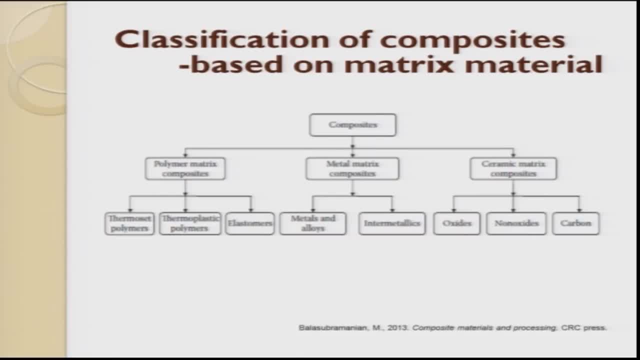 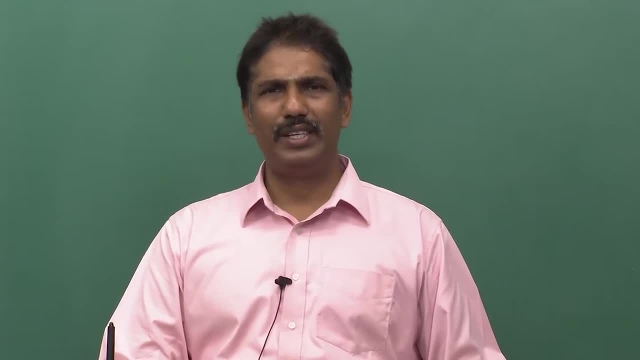 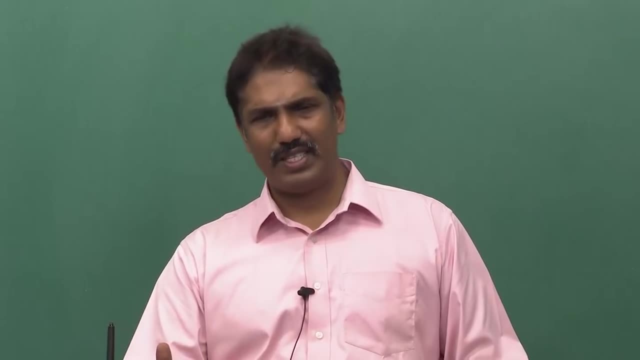 used in ah mankind today. So the next one is metal matrix composite. metal matrix composite are used where in which there are high strength and you need more high strength materials and more other properties like stiffness and corrosion resistance- all these things we are now trying to add metal matrix composites there. 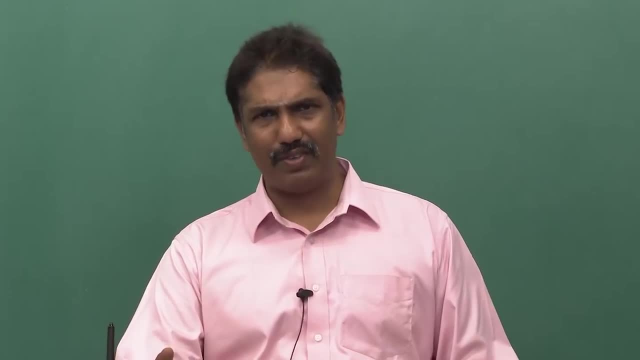 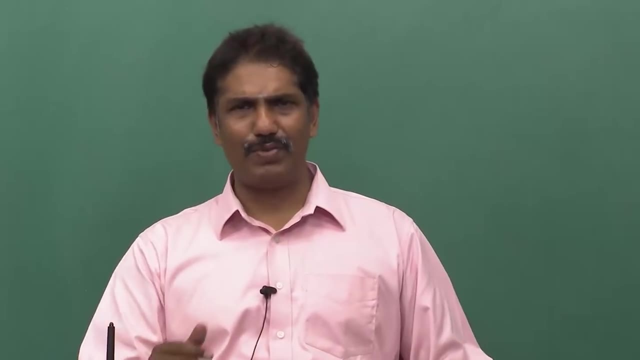 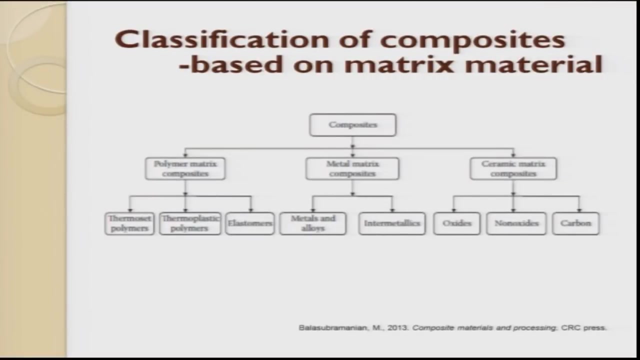 So metal matrix composite ceramics are very poor in toughness, So now we add reinforcing agent to enhance their toughness property. Same way with metals: we add reinforcement so that we enhance their strength property. When you talk about polymer matrix composite, they are further classified into three. Generally there are three types or three kinds in polymer. 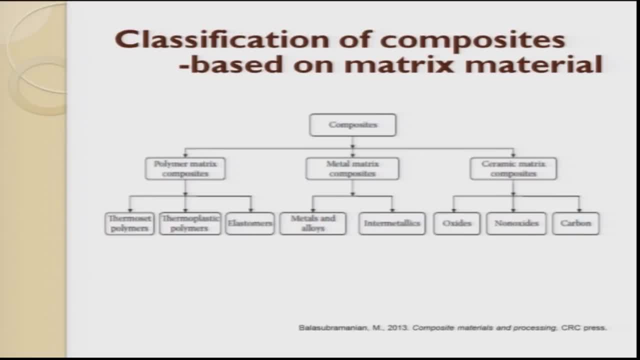 one is called as thermoset polymer, another one is called as thermoplastic polymer and the third one is called as elastomers. Thermoset polymers are polymers where in which it has very high strength and stiffness but, as far as ductility is concerned, is very poor, and 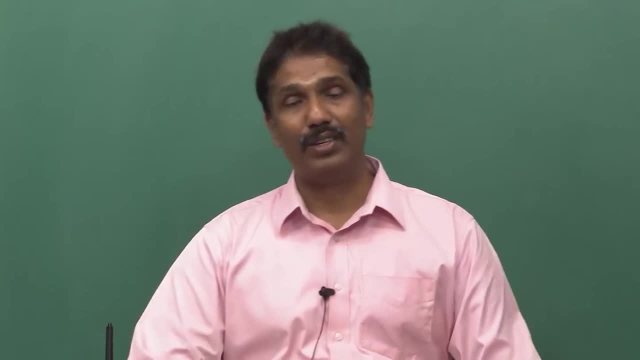 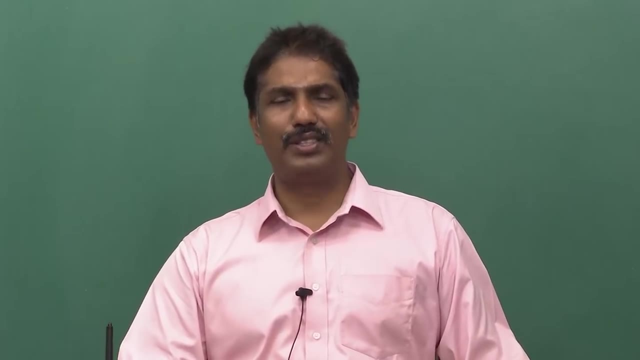 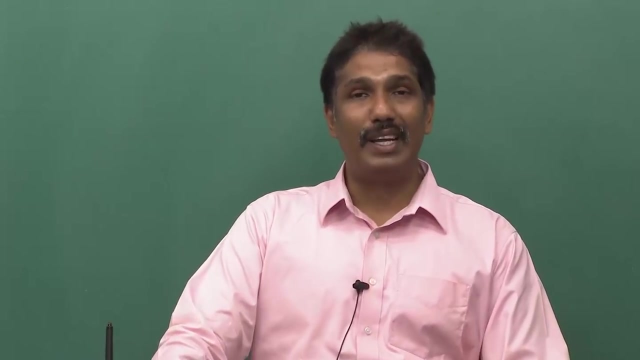 on top of it. these composites are not recyclable. Today, there is a major challenge which is thrown in front of us is how do we process the thermoset polymers which has been installed in service condition in the last few decades, Thermoplastic polymers. these polymers are recyclable. they 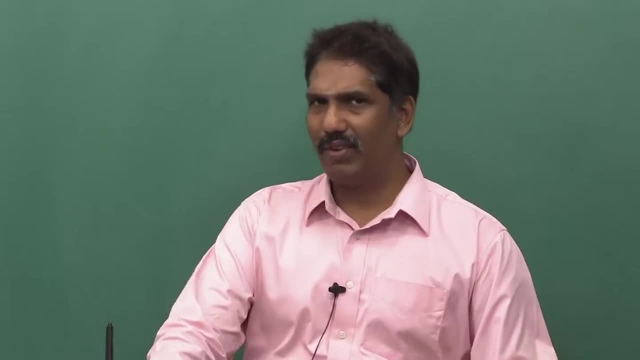 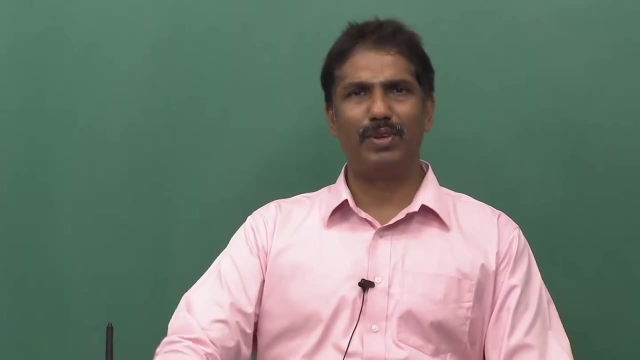 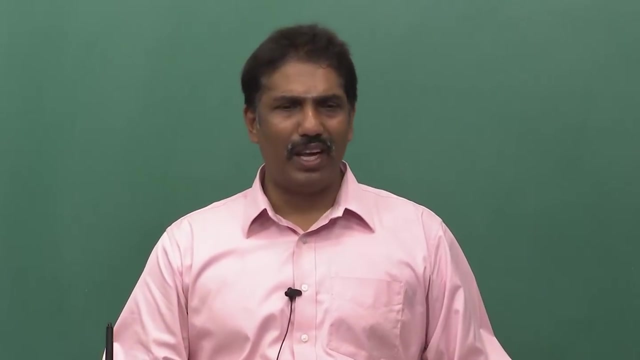 have strength, they have also ductility. The major advantage of thermoplastic is recyclable. Today there is a new offshoot of polymer- thermoplastic polymer, which is coming, which is called as biodegradable polymers. They are slowly gaining importance. however, they have not gone into. 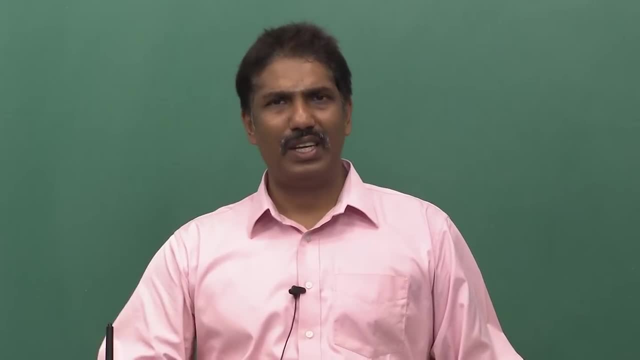 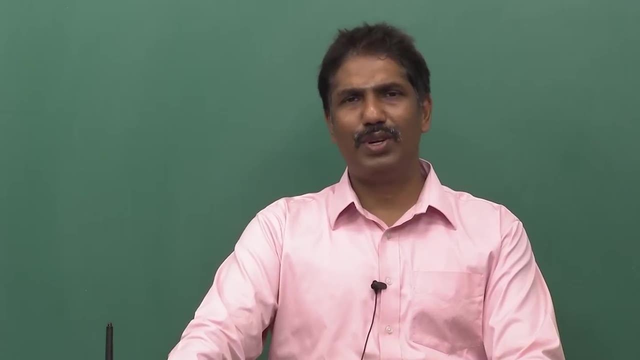 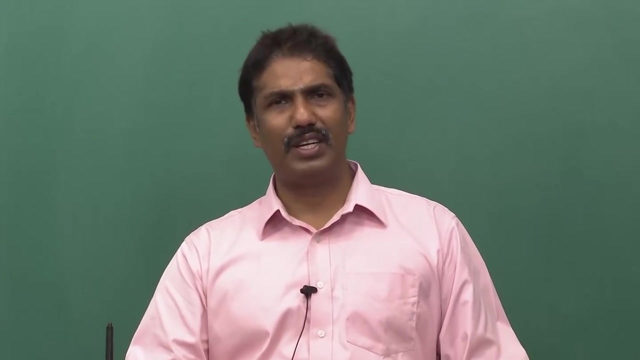 the application of strength stiffnessrequirements. The last one is elastomer. elastomer is also part of polymer. The difference between thermoplastic and elastomer are: elastomer has a ductility from 100 percent it can go up to even 2000 percent. the elongation can happen. Simple example is your rubber band. 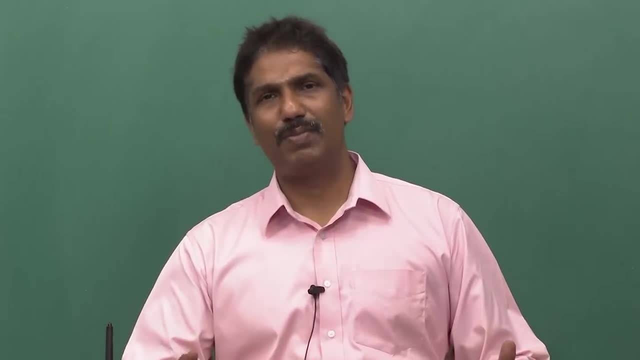 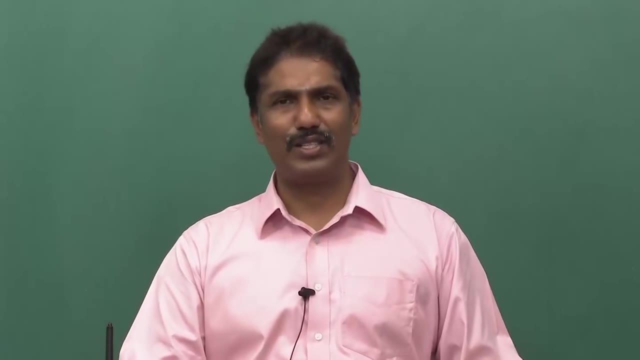 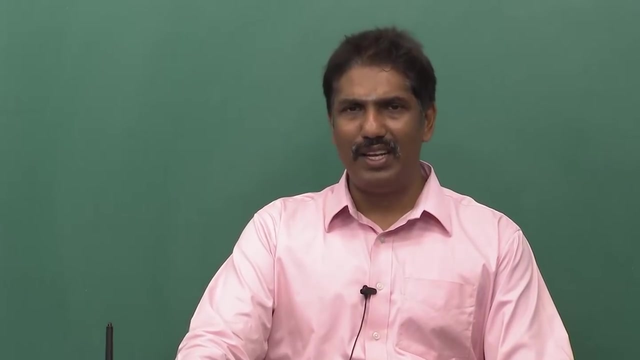 the thermoplastic elastomers. you can see a wide spectrum of application, right from a rubber band to a cycle tyre to a plane tyre. all these things are elastomers based composite materials. We always try to reinforce with steel and carbon fibres to get the required properties. 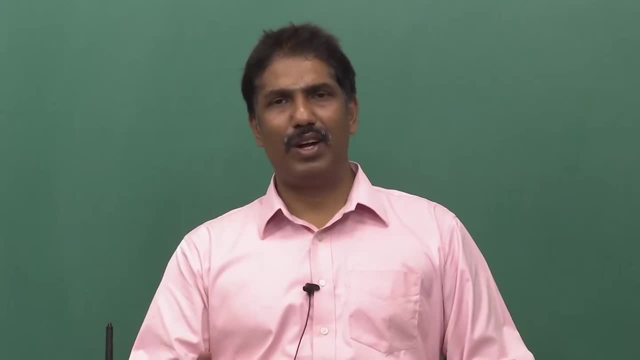 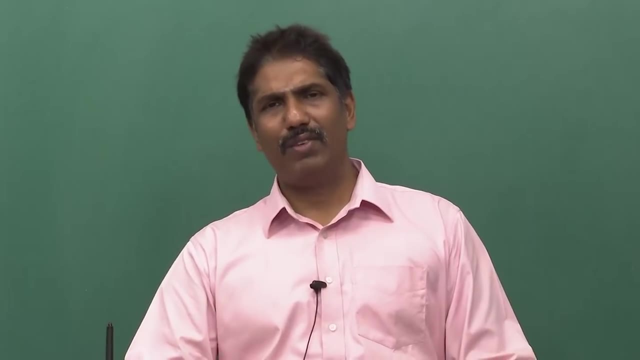 When you go for metals, we take two kinds in them. one is called as metals. you can take pure metal, try to mix it, or you can take an alloy and try to mix it. predominantly, whenever we talk about strength, we always talk about metal alloys getting mixed with a reinforcing. to match out the requirements. So here again strength versus weight ratio is taken, and here there are found to be major advantage. One good example: today what is happening is the huge electrical transmission towers are made out of ah metal matrix composite. today The copper wire, the cable which carries very high current, are now made out of metal matrix. 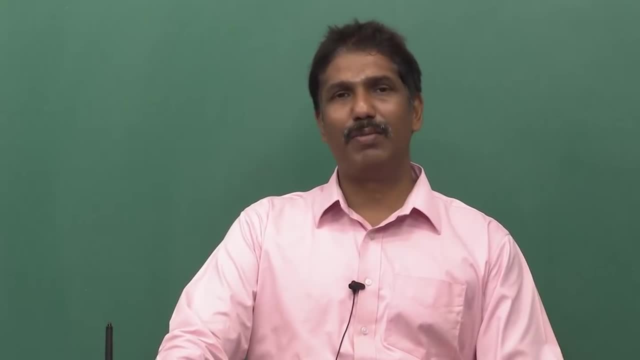 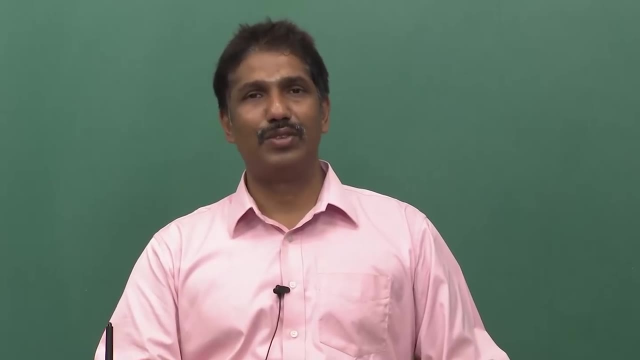 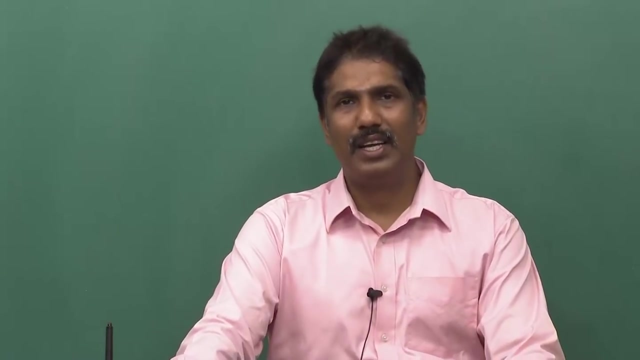 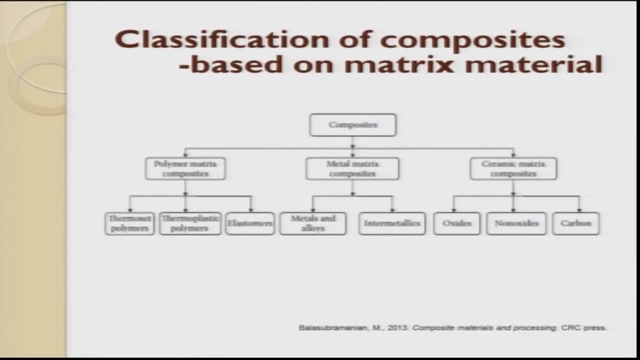 composite. because of this coming of metal matrix composite wires, the sagging happens low. the number of towers for reinforcement has also reduced. This has given the transmission industry a huge boom. Next is intermetallics. intermetallics are an offshoot of metal matrix. here the alloys occupy a fixed stoichiometric ratio, and this 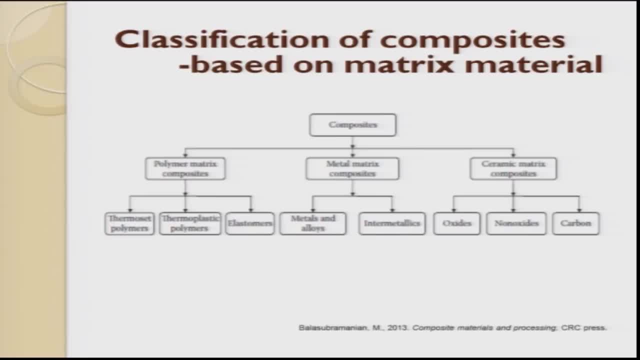 intermetallic composites are used for high temperature applications. When you talk about ceramics, there are three classifications: one is oxide ceramics, another one is non-oxide ceramics and the third one is carbon. When you talk about oxides, I am talking about. carbon. 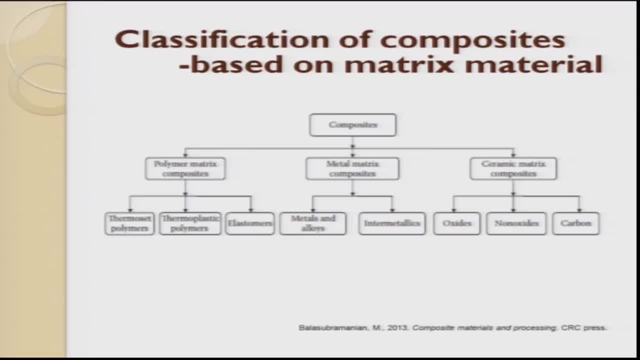 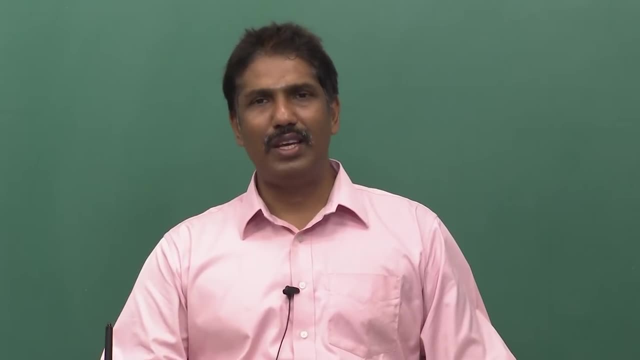 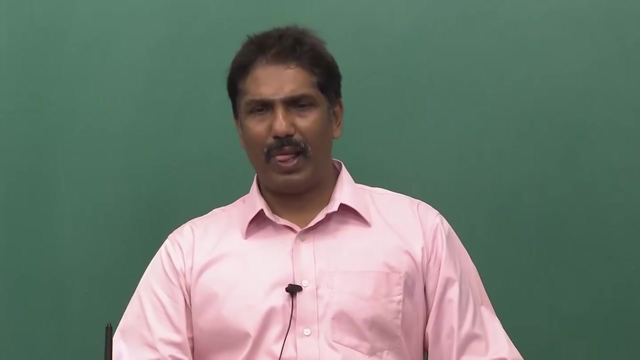 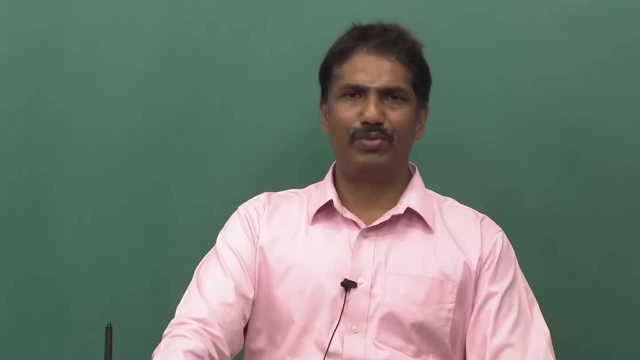 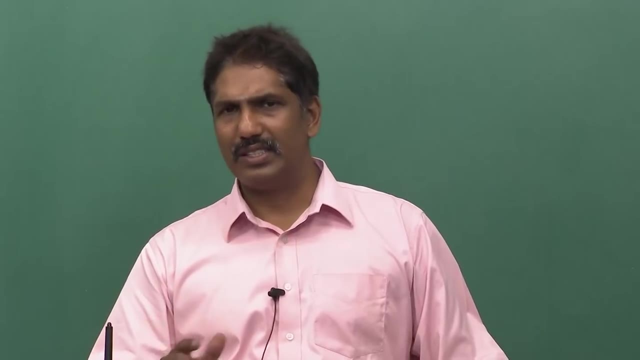 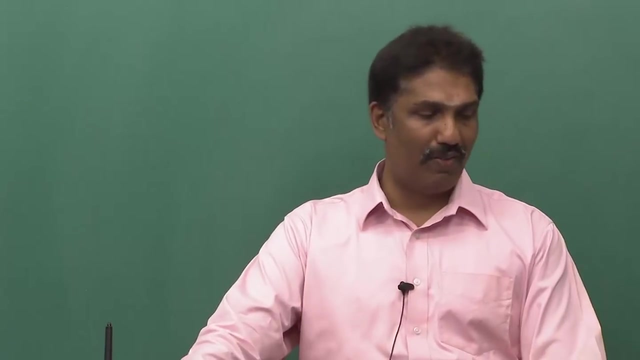 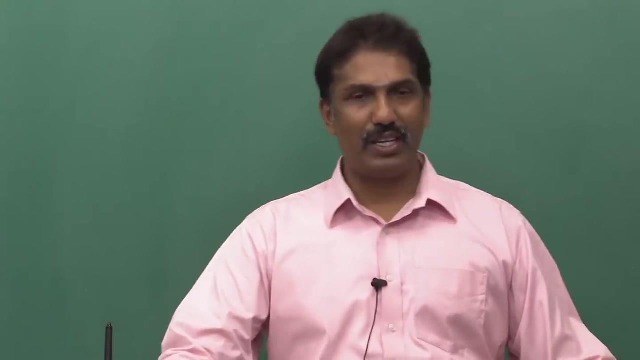 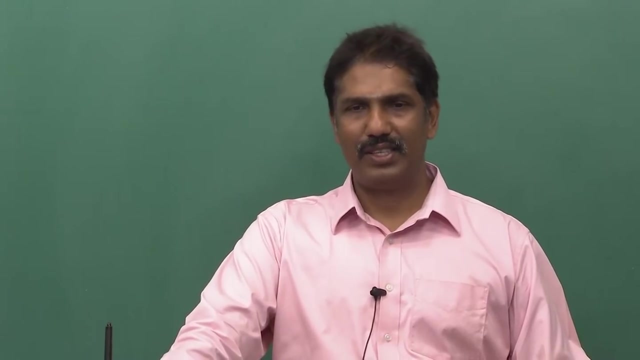 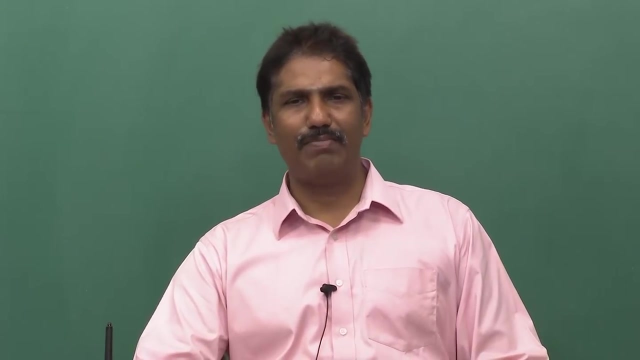 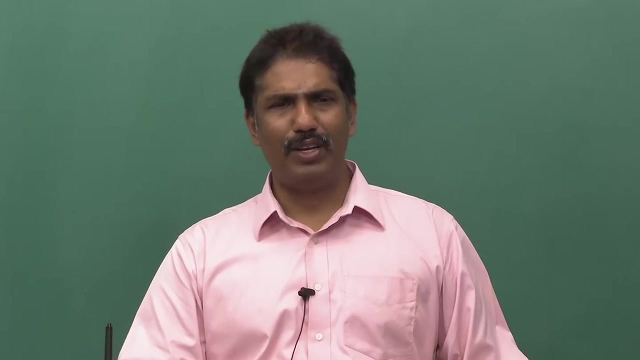 about matrix phase. Now let us see some of the properties of the composite when I when I compare it with that of metal. So I take only two metals for for because these two are commonly used. one is steel, the other one is alumina. So if you see a weight, wise steel. 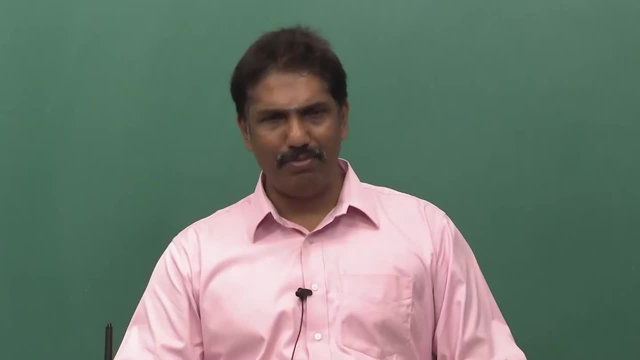 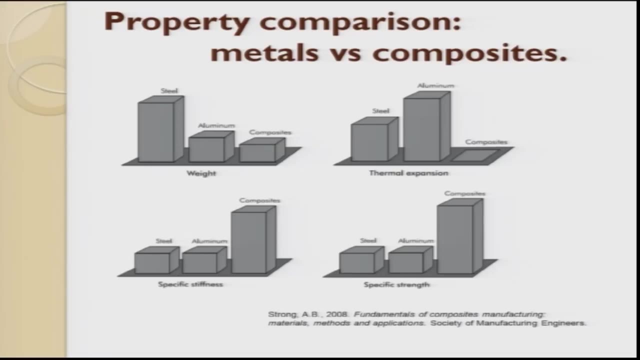 has a very high density. followed by it is alumina aluminium. So this aluminium is nowadays getting replaced wherever steel was used. and second, aluminium has an advantage of corrosion resistance. So aluminium is now playing a major role Now when we move towards composites. 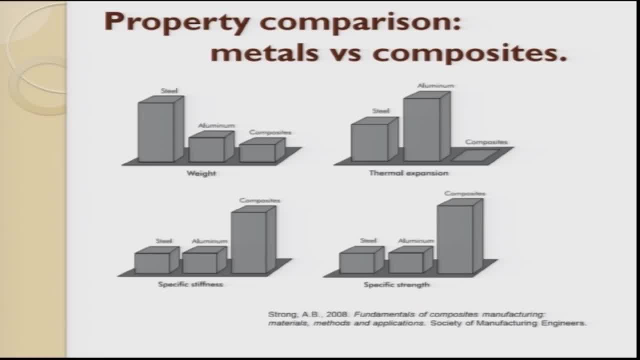 it is much lighter than even aluminium. So if you have a moving body and if you want to have a better efficiency of of mileage, then we replace that aluminium also by composite materials. So next one is thermal expansion. you see, thermal expansion of 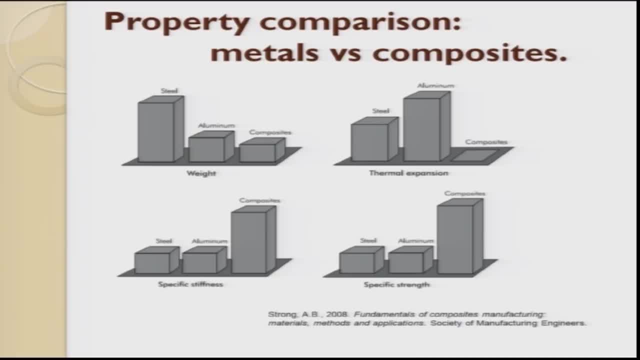 Steel is much better than that of aluminium, but when I try to make a composite it is almost close to negligible. When I talk about stiffness, it is also seen that steel and alumina are very close by. composites have a very high specific stiffness, Then with specific strength, 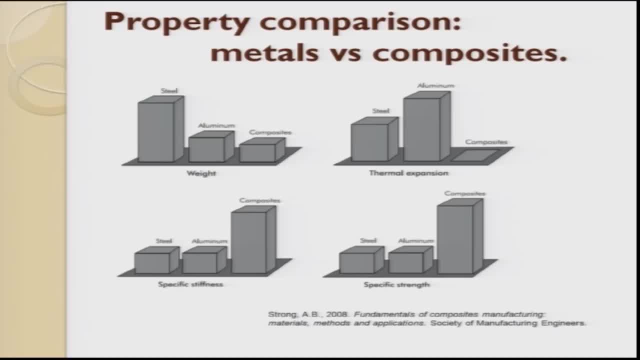 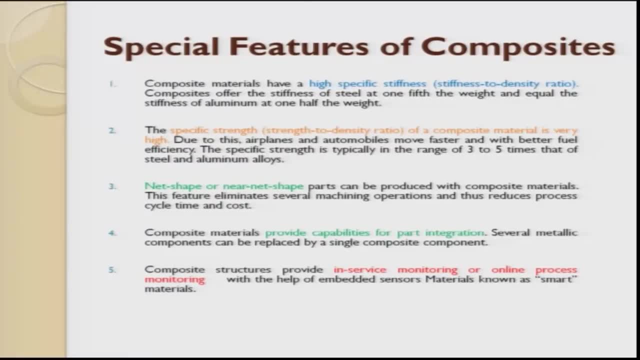 the composites excel out with this. let us see move further and see what are all the special features of composites. So the composite materials are materials which have high specific stiffness. What is high specific stiffness? Stiffness to density ratio, So stiffness divided by density. So 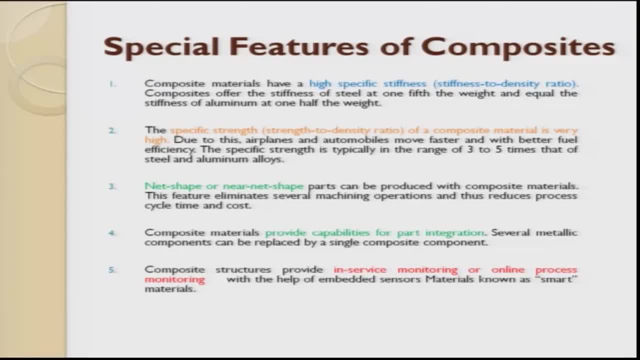 this will try to give an advantage and see what is the weight I have to add to get a required stiffness. ok, The next one is with respect to strength. Stiffness and strength are two different properties. Please make a note: people interchange- unknowingly- stiffness. 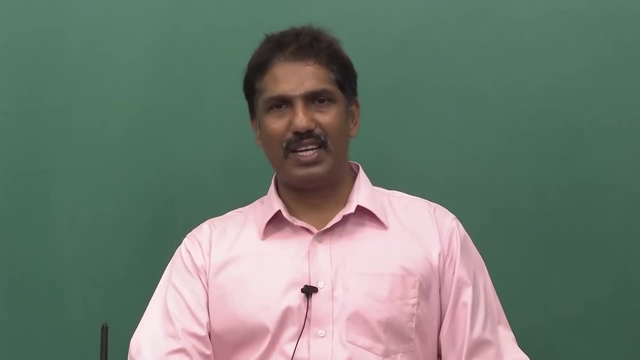 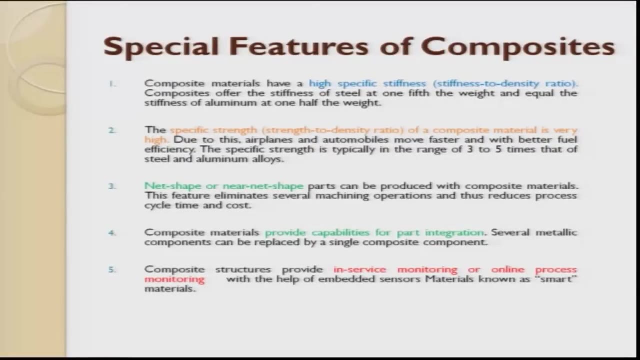 is different. strength is different. Stiffness is taken in the elastic zone and strength we always take in the ultimate strength, and we talk about that. Next one, composites are those materials which can be made up to near net shape Today in manufacturing the entire. 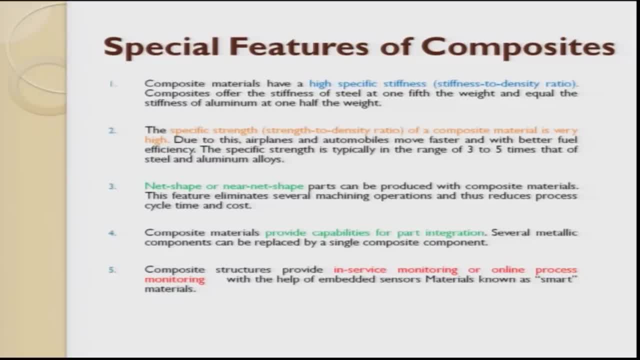 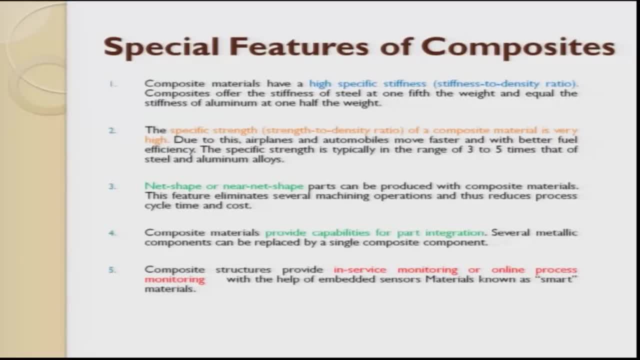 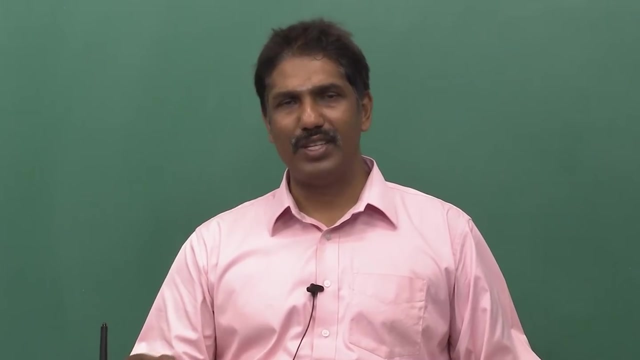 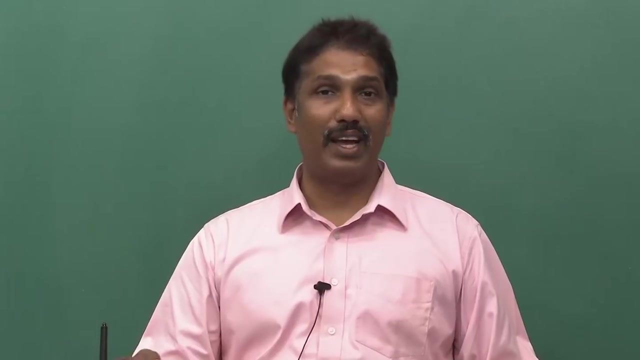 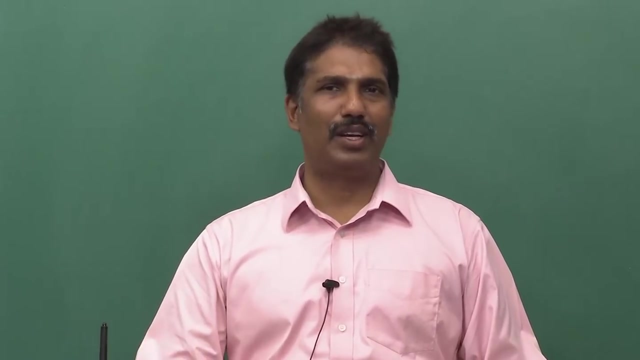 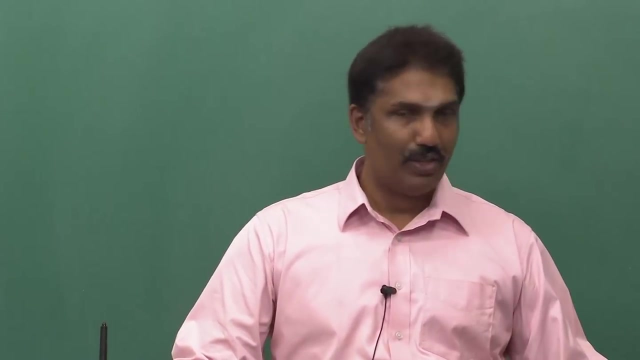 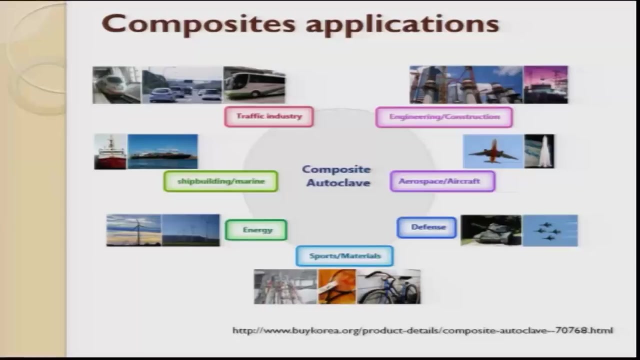 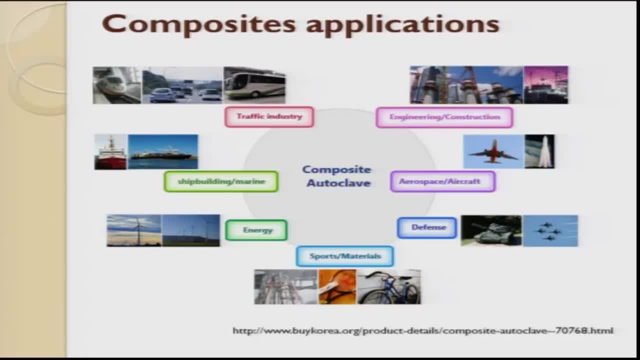 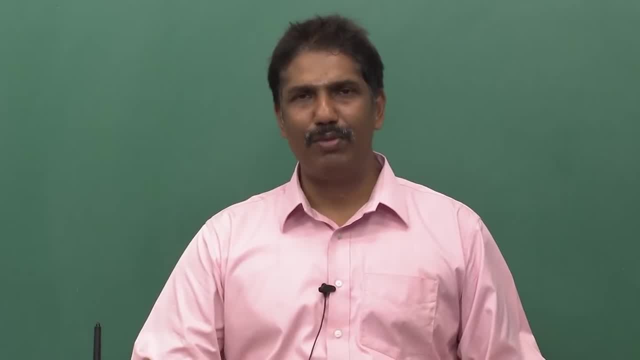 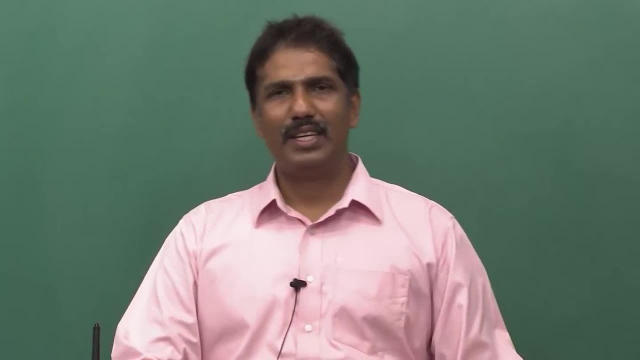 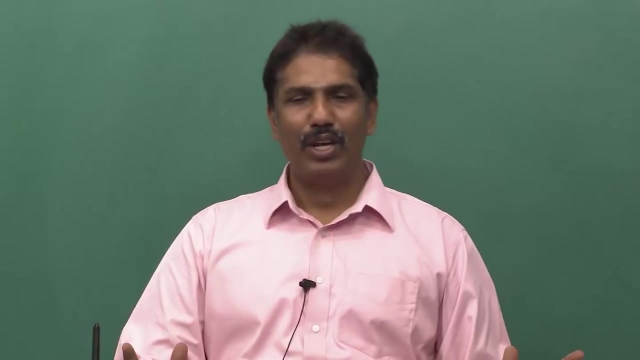 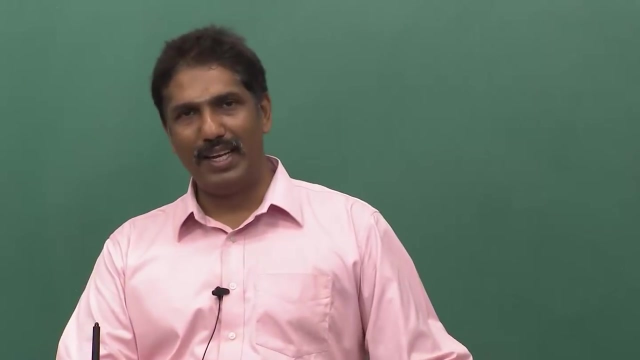 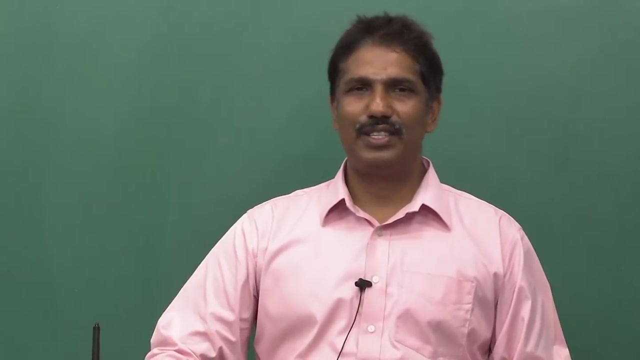 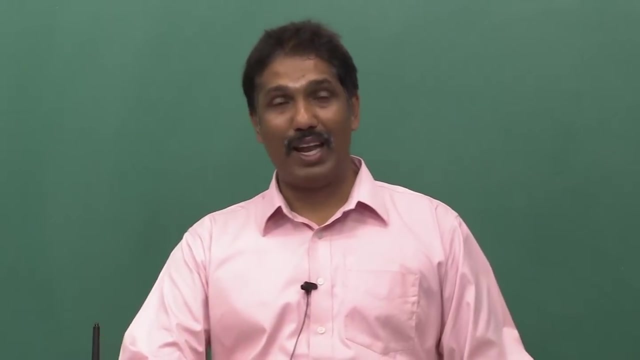 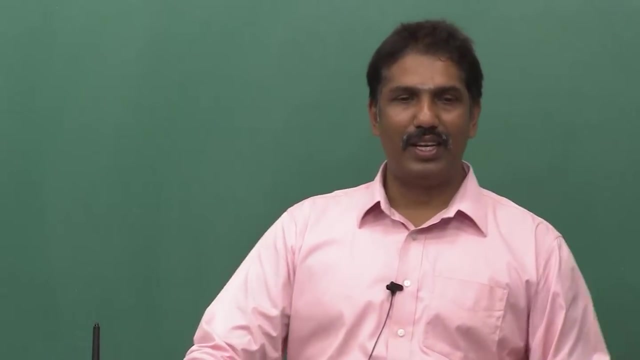 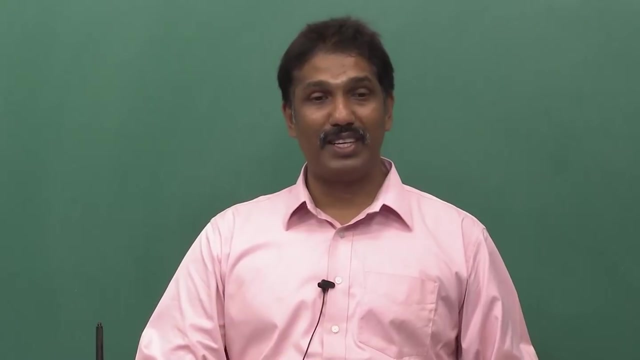 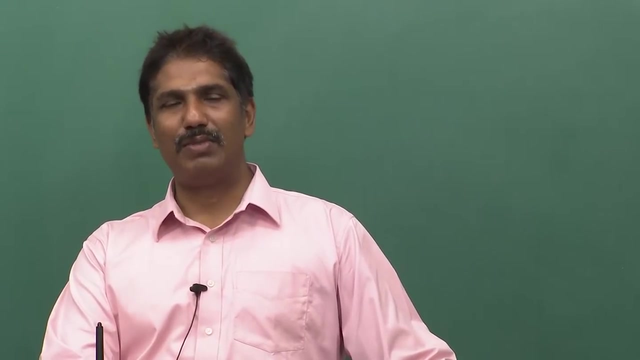 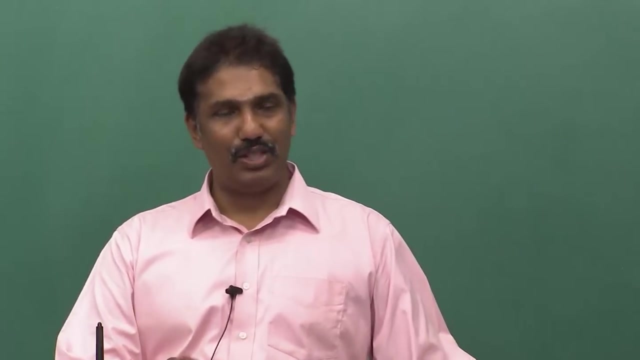 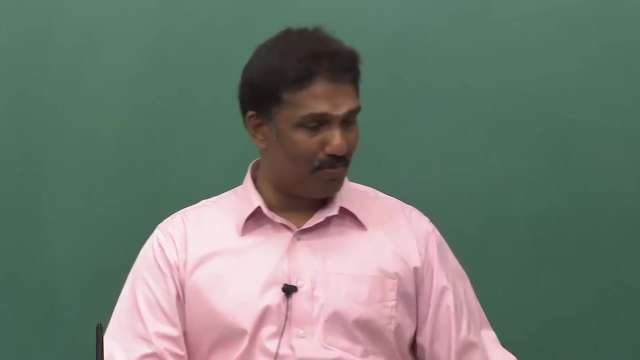 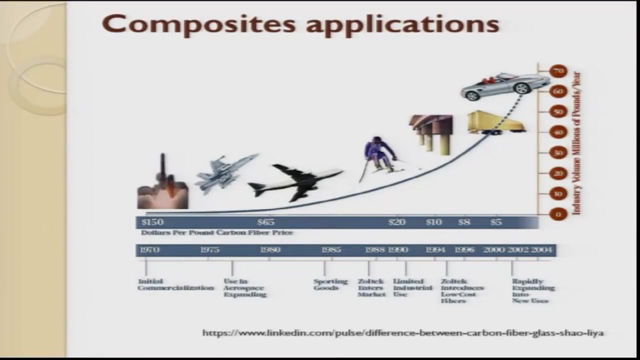 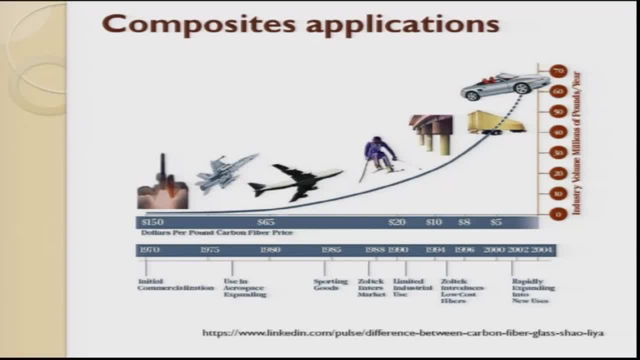 So you can see, the usage of composite materials in various industries have enhanced, and also the amount of money which is getting invested in millions of pounds per year is shown in this graph. This is a old graph- 2004- and the graph keeps exponentially increasing, even today for various 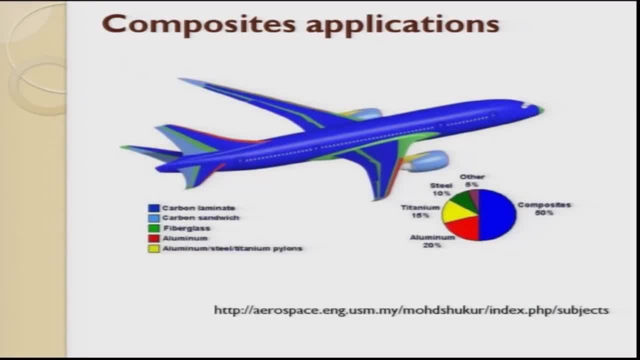 applications. So when we take a commercial aeroplane there are about 50 percent of the material is made out of composites. I will repeat: So it has very high strength to density, stiffness to density. it is made up to near 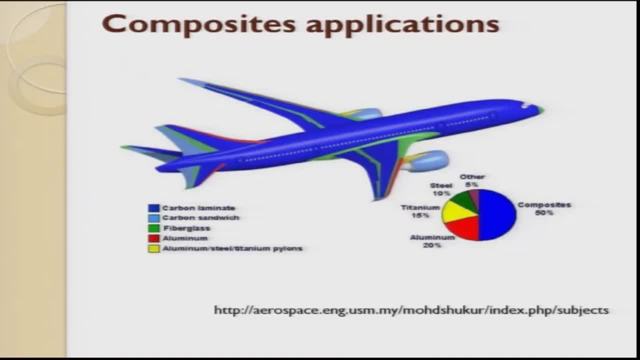 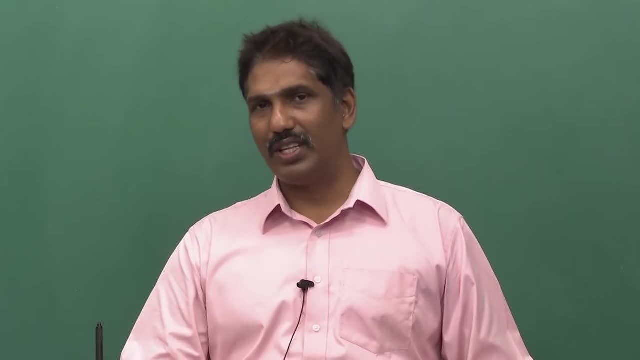 net shape So I can give a aerodynamic profile very easily. I can integrate with other parts very easily. So when I want to do part integration, composite comes up in a very big way. So today, from 50 percent of the composites, people are now stretching themselves to go. 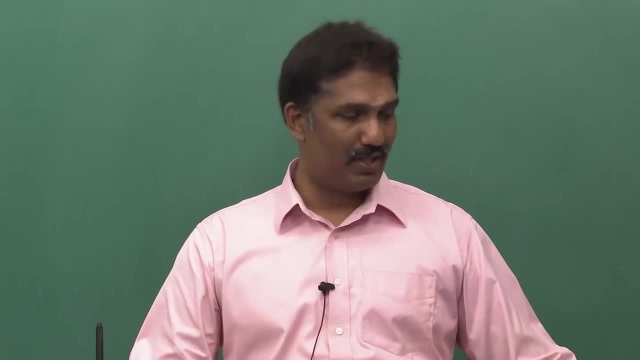 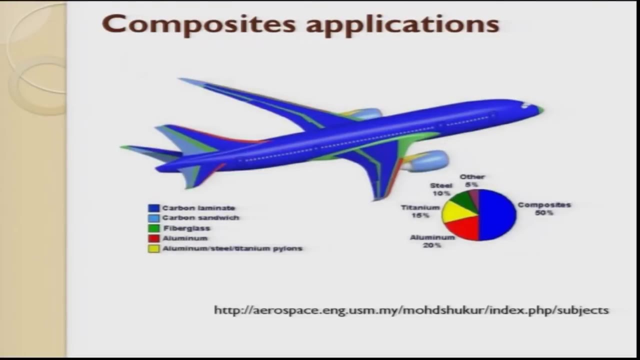 up to 75 percent made out of composites. So here I will show the structure which I have different, different color codes. I am sure it is visible for you. We have people have started using carbon composites. people have started using carbon sandwich. 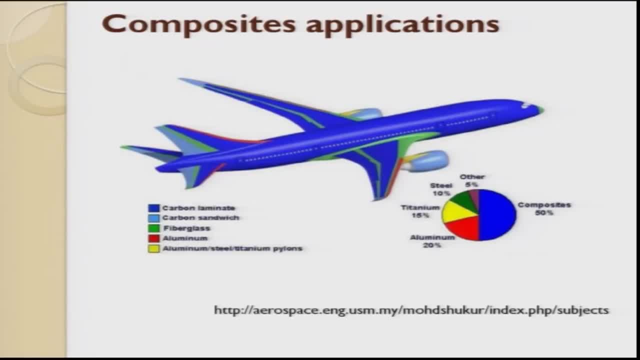 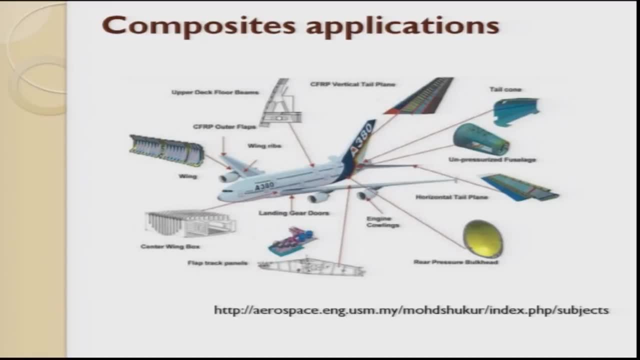 composite. We will see what is sandwich later- Fiber glass and they have also started using aluminum metal matrix composites. So these are some of the parts which are used which are made out of composites. For example, CFRP. vertical tail planes are there? tail cones are made out of it. rear 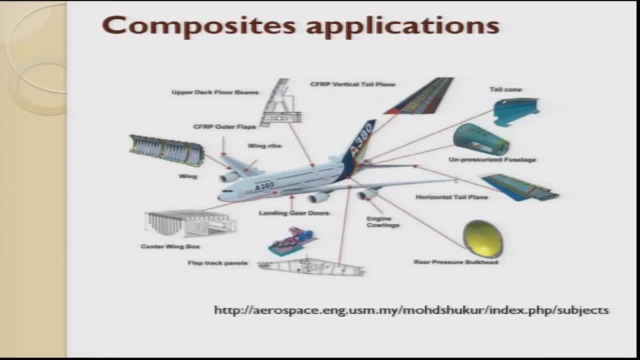 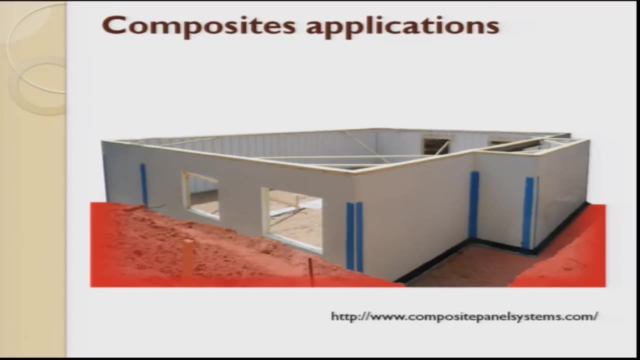 projectors are there. Rear pressure bulk head is made out of composites, injured cowling is made out of composites, wings are made out of composites and center wing box is made out of composites. Today, houses are made out of composite materials and these houses are first it came into existence. 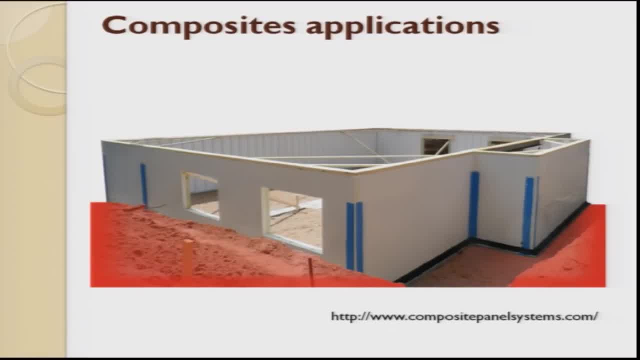 for disaster management. but today what has happened is rapid construction are required in the third world countries. So here the complete the roof. complete roof and the side panels are made out of polymer matrix composite which has acoustic proof plus. it also has part integration with steel. 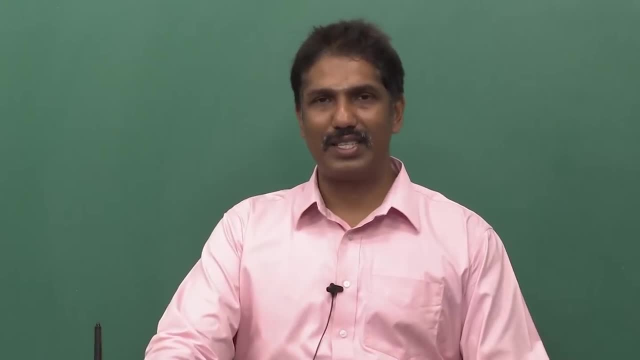 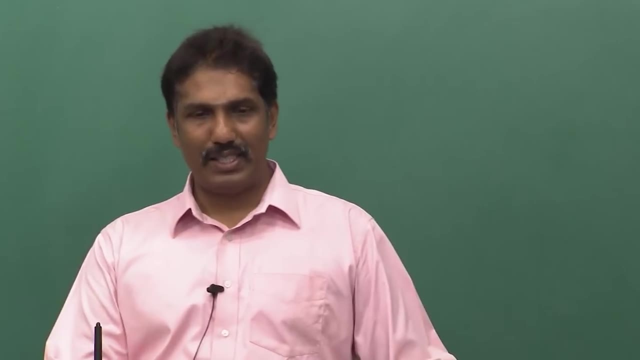 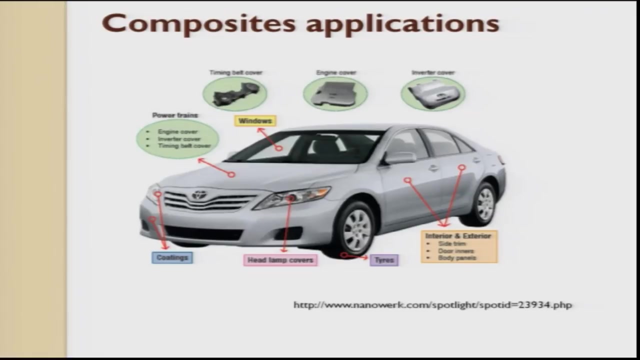 fasteners So you can quickly go assemble it at the required site and it it gives a big boon for the construction industries. Cars, as I told earlier today, in cars also there are lot of parts which was earlier made out of alloys, Because alloys are getting replaced by metal matrix composite materials for making the 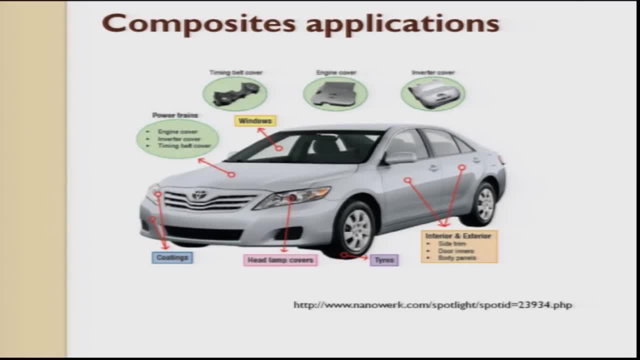 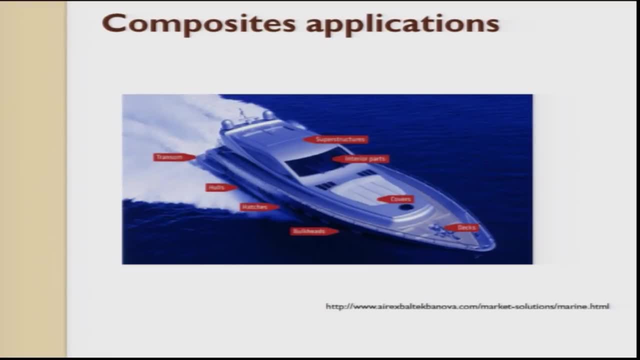 car lighter, stiffer and perform much higher. Mar 자� Immeril industry, where corrosion is a big problem. So here the superstructure, interior parts, cover, deck, bulk, head, hatches, hull and transforms- all are made out of polymer matrix composite. 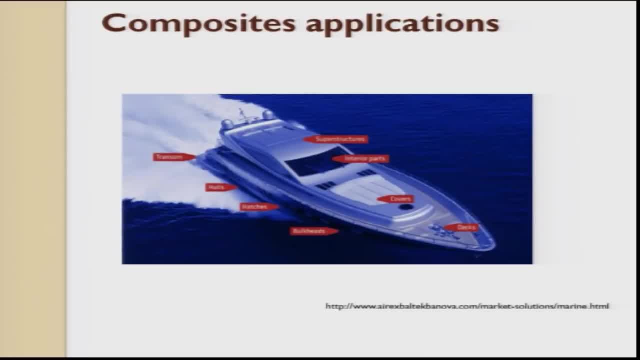 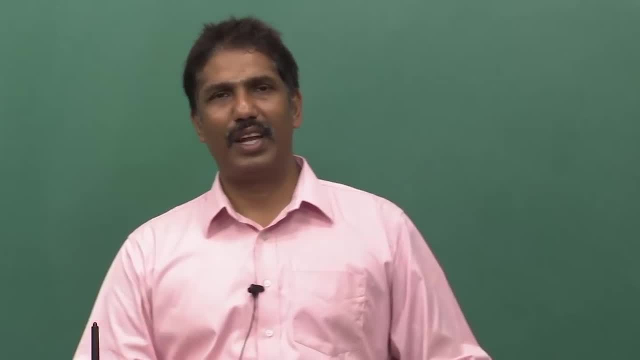 So again here, When you make composites- 24 بّURE เสิ้mania久- you have to look at two things. one is called as primary structure, another one is called as secondary structure. In primary structures are structures where in which predominantly 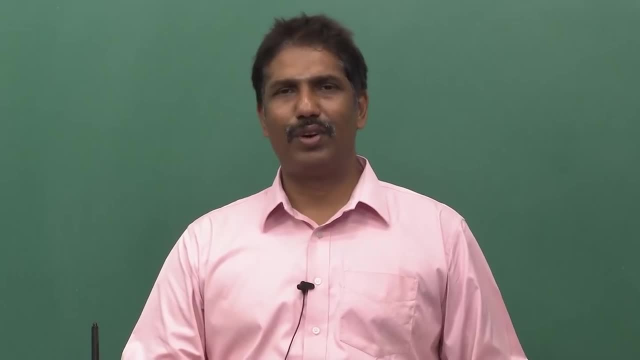 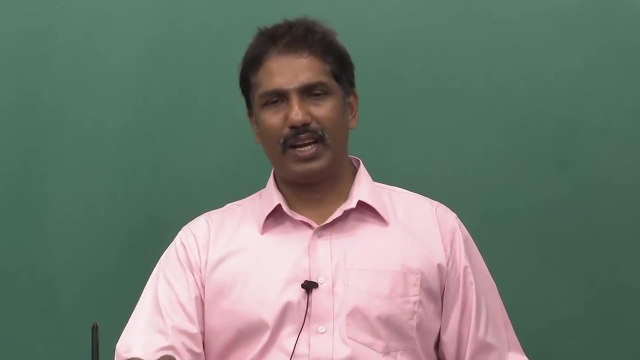 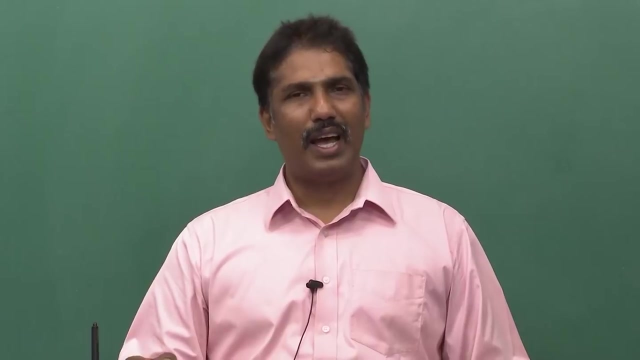 it takes load. Secondary structures are used for filling, for giving other secondary properties which are required for the product. So when you take a marine application of composites, there are lot of primary structures made out of polymer matrix composite as well as secondary structures made out of polymer matrix composite. Simple example for secondary structure is: 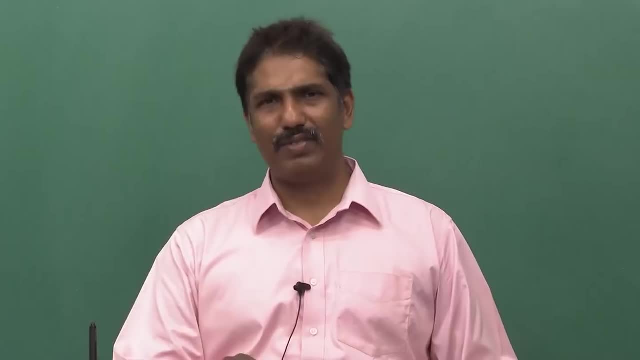 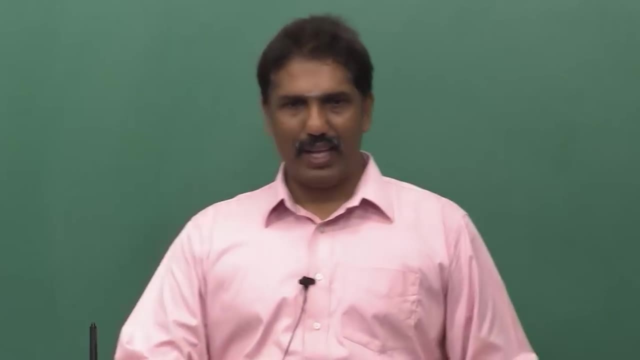 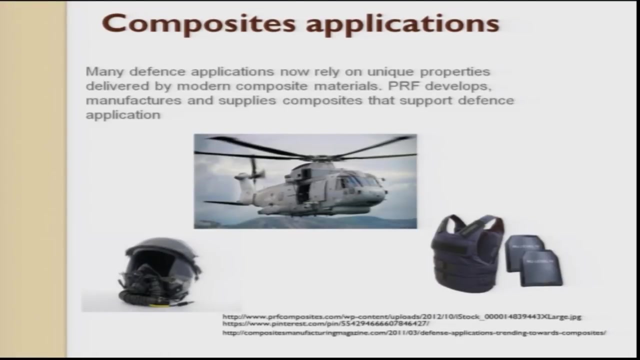 deck where in which it is. it is only a spacer where in which it is used for the movement of human being around. As I was talking to you about, defense, helmets have become much lighter. bulletproof jackets have become much lighter, but lighter and high performance. So in inside a bullet jacket, now ceramic. 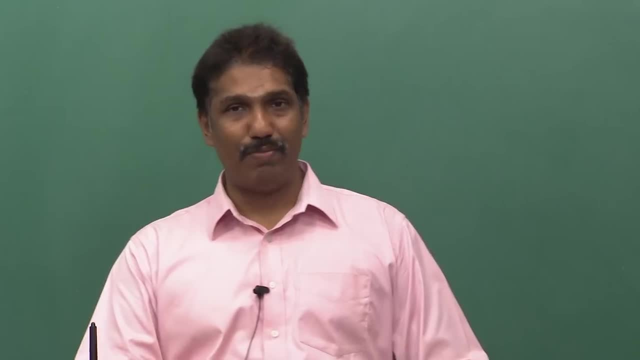 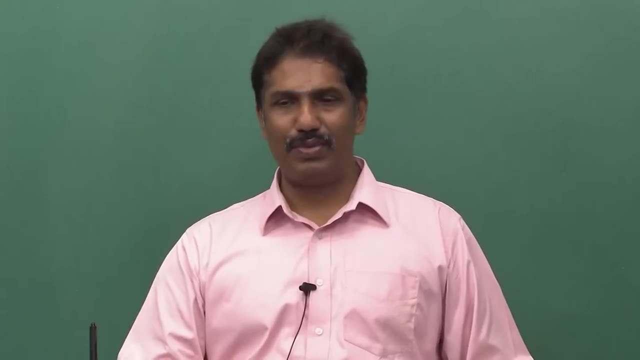 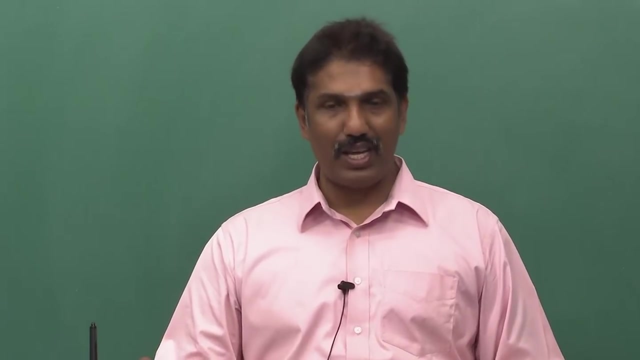 tiles Are used. these ceramic tiles are again a composite material which has very high toughness and very light in weight, So which helps the soldier without getting fatigue when he is in operation, he can perform efficiently. The helicopters are made out of carbon fiber reinforced. 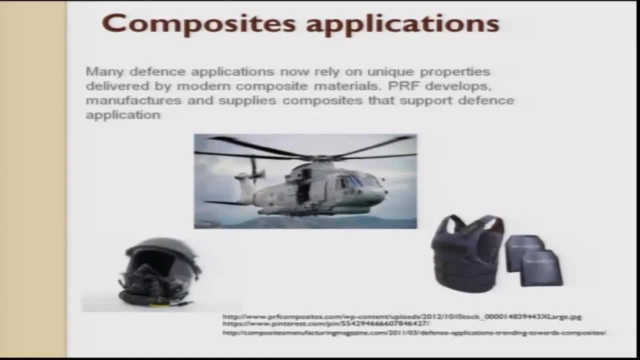 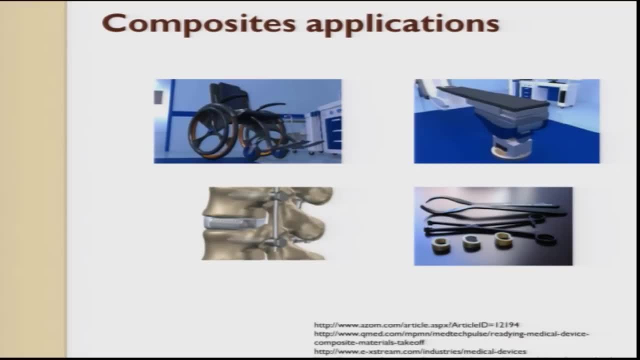 composites: the the blades of a quadcopter or a helicopter are made out of light weight materials So that it gives stiffness as well as Weight is less in. in biomedical applications there are lot of products which are coming out which is made out of composites: wheelchair is one, and then you see lot of appliance which 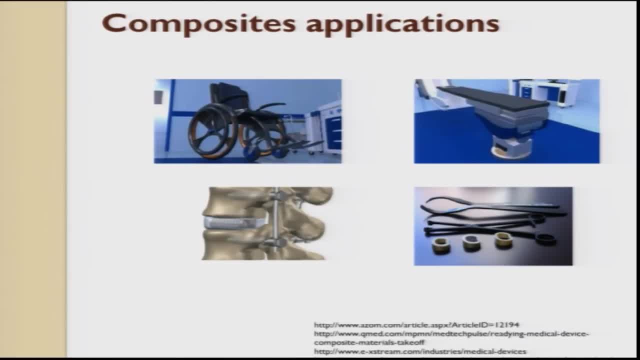 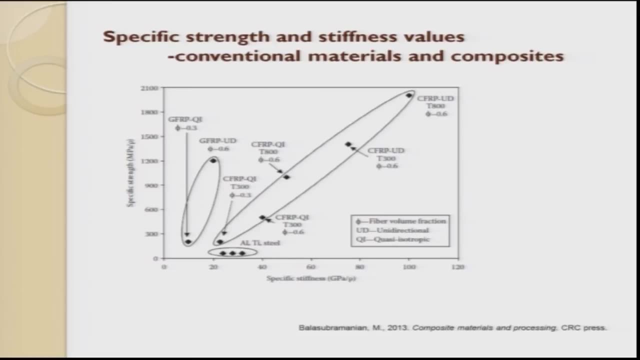 are are the fixed lot of fixtures and apparatus are made out of composite metal matrix, composite material, So that they perform high or they perform good. So, in a nutshell, if I want to put plot between specific strength to specific stiffness, As I told earlier, these two properties, 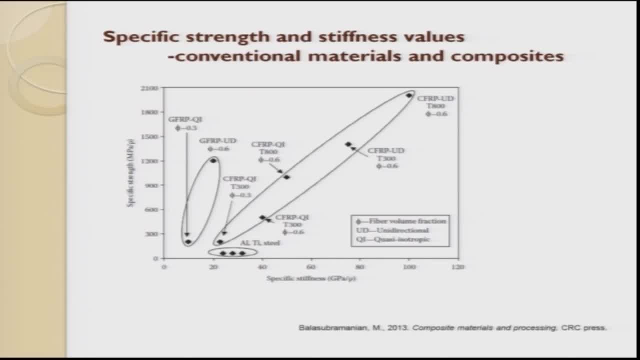 are different: stiffness versus strength. If I draw a plot, you can see in this plot I have accommodated glass fiber reinforced composite, carbon fiber reinforced composite, So you can choose which one to pick. you can choose and pick what is required depending upon your 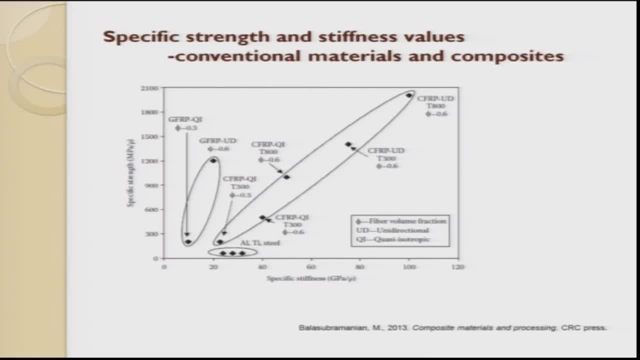 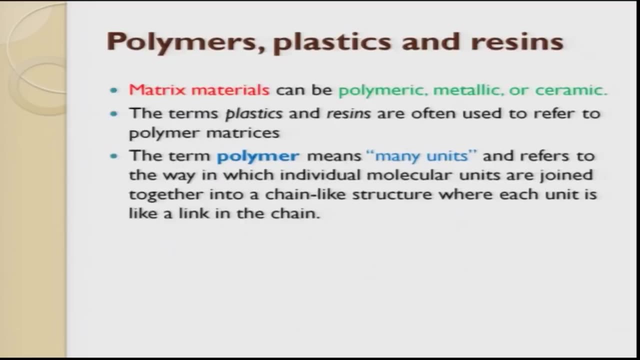 application. So you look at conventional materials- aluminum, titanium, steel- look at their specific strength to stiffness ratio and look at carbon fiber reinforced plastics- unidirectional the strength versus stiffness value. So now let us get into polymer. So polymer is otherwise called as plastics, and when it 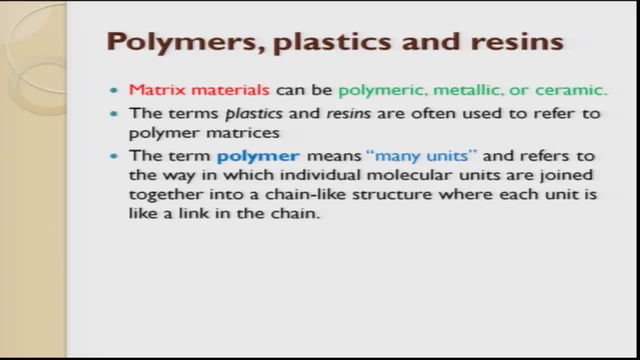 is used for fabrication, it is called as resin. So the name polymer clearly tells that the there are lot of monomers joined together to form a polymer, So the matrix material can be polymer metal or ceramics. but from now on, for the next few lectures, we will focus. 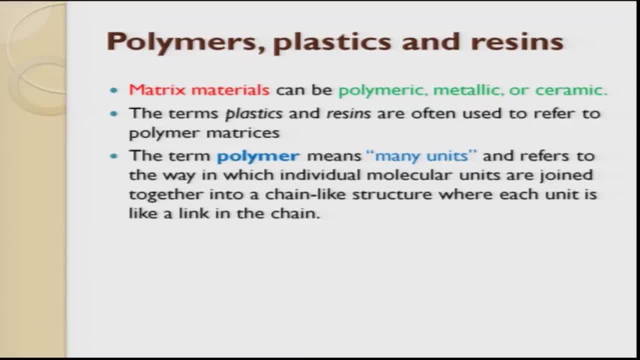 only on polymer matrix composite. The term plastics and reinforcement are often used to refer polymer matrix composite. The term polymer means many units are joined together and form a chain And this chain, like structure, will try to will. this chain, like structure, is called as polymer and inside this polymer we try to add reinforcement and make a composite material. 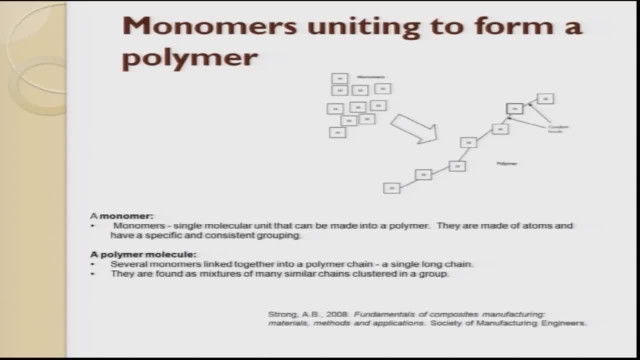 So these are schematic diagram. you see lot of mers which are dispersed and these mers join together like a chain. So the mer is nothing but a bead in a chain, all these beads which are nothing but a bead. So these beads are nothing but a bead. So these beads are. 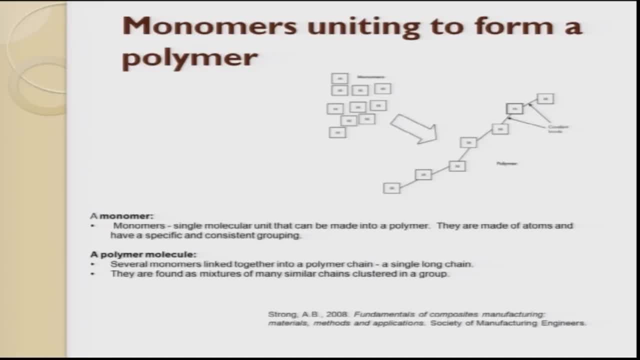 nothing but monomers are joined together to form a wonderful chain and this formation is called as polymer. A monomer is a single molecular unit that can be, that can be made into a polymer. So a monomer is made out of atoms and have a specific and a consistent. 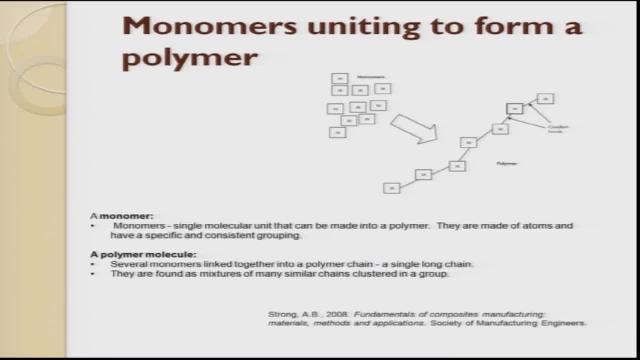 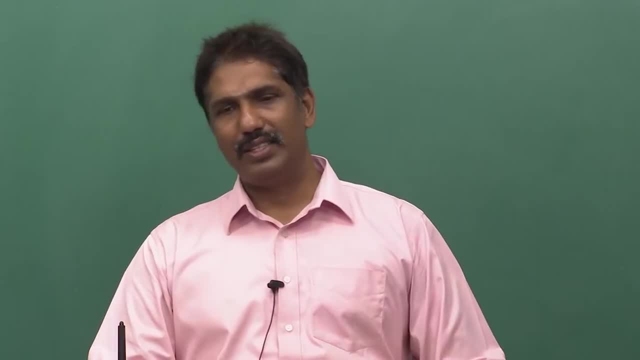 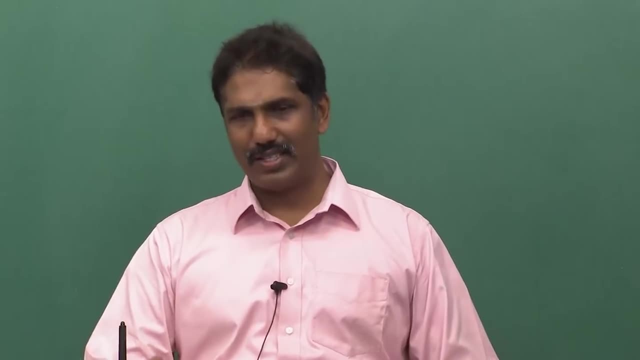 grouping. What is a polymer? A polymer molecules are nothing but several monomers linked together to form a polymer chain. It has a single long chain. The single long chain alone cannot be used for applications. There will be several chains attached together and there will be forming clusters and this clustering of monomers into 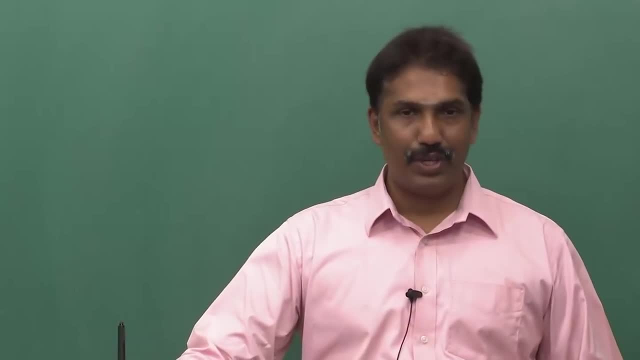 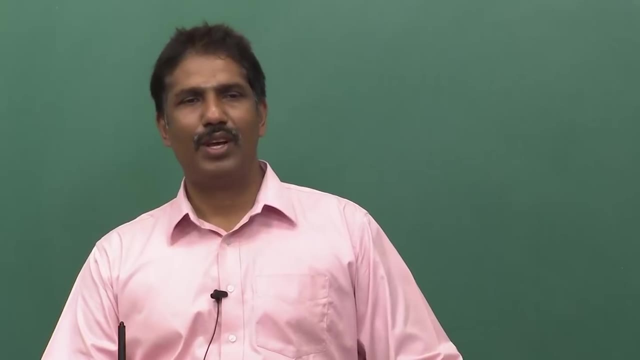 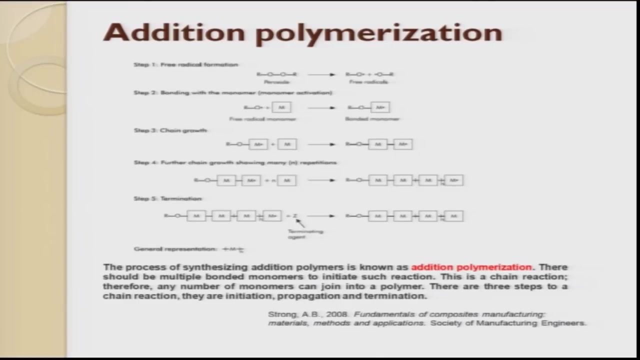 a chain fashion is called a polymer. So there are two basic mechanisms which are involved for for this polymerization process. One is called as additional polymerization, the another one is called as condensation polymerization. In additional polymerization there are 5 steps. 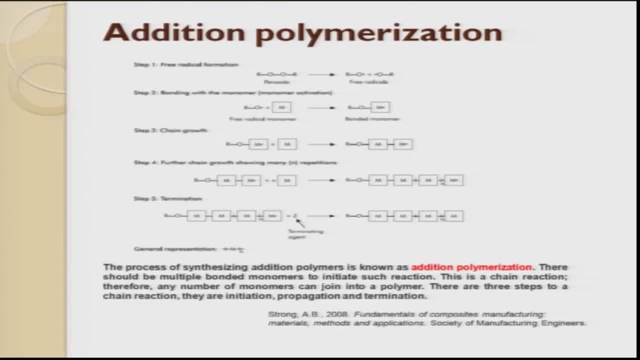 involved. So the 5 steps are: first the free radicals are formed, then, bonding this, the formed free radicals try to bond with the monomer, and then this monomer tries to join with each other. they form a chain. and this chain keeps on further multiplying and growing, and this 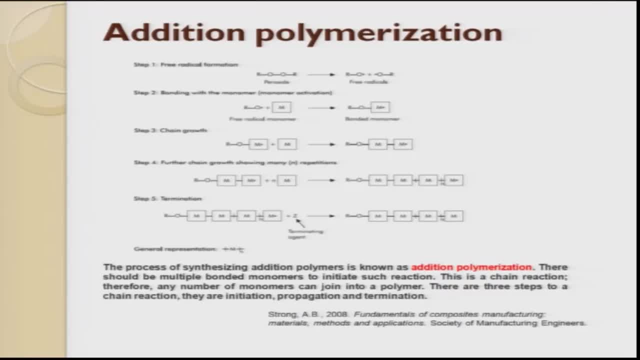 cannot keep growing for infinity period. So there will be something called as termination step, so that it terminates the polymer. So if you want it, it is a simple analogy- is: I have a set of beads, So all these beads are there in a box. these beads have to be linked to each other. how do we link with one? 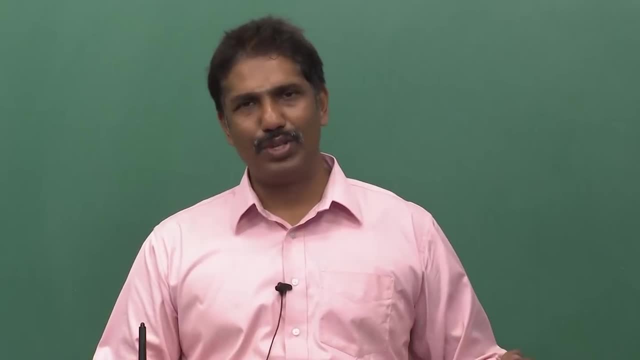 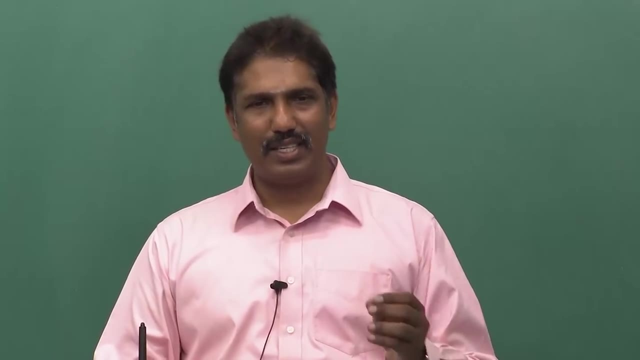 we apply a adhesion and stick all the beads. the other way around is we use a twine which can pass through all the beads and form a chain. It is almost the same thing. the radical is which is, which is a peroxide, which which forms free radicals. these radicals get attached. 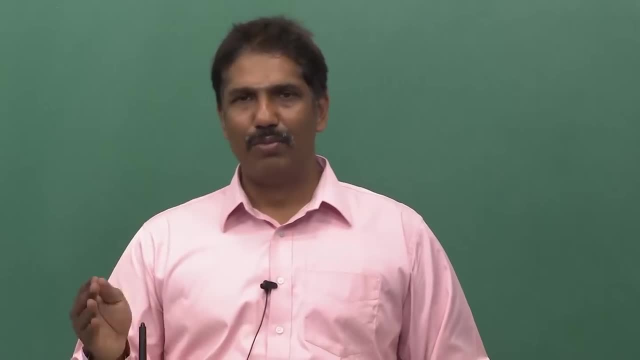 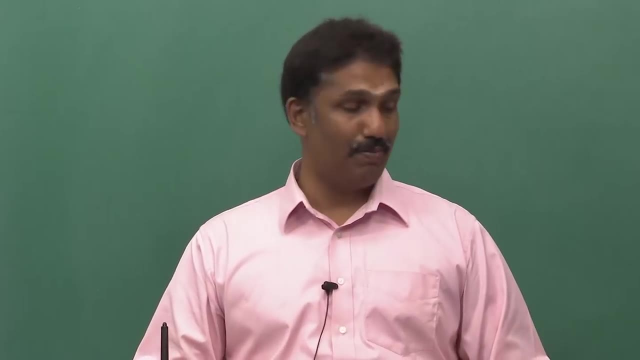 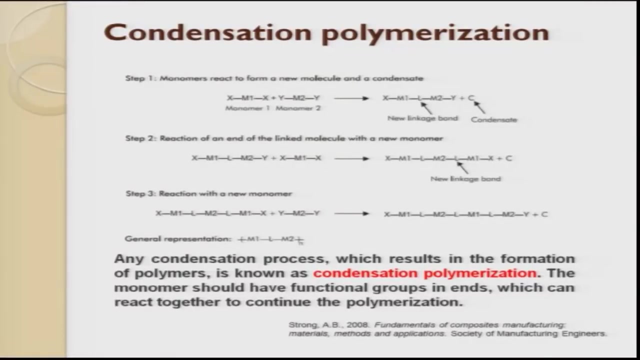 to the monomer. So monomer gets attached to monomer, monomer, monomers, monomers get attached and then finally they get terminated. this mechanism is called as adhesion polymerization. The next mechanism is condensation polymerization. in condensation polymerization what happens? the monomer reacts. 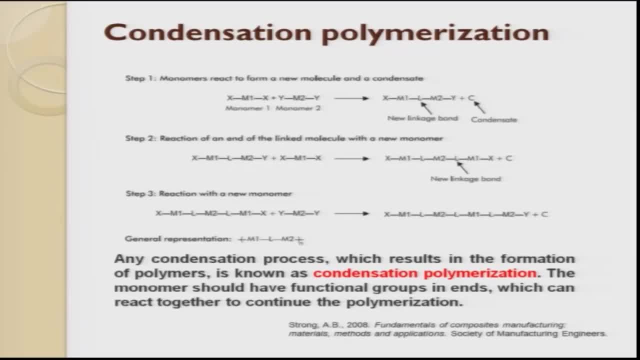 to form a new molecule and a condensate. the condensate is predominantly nothing but water. So it is you have this monomer joining with another Monomer. when these monomers join together, form a link, they also form a condensate. So 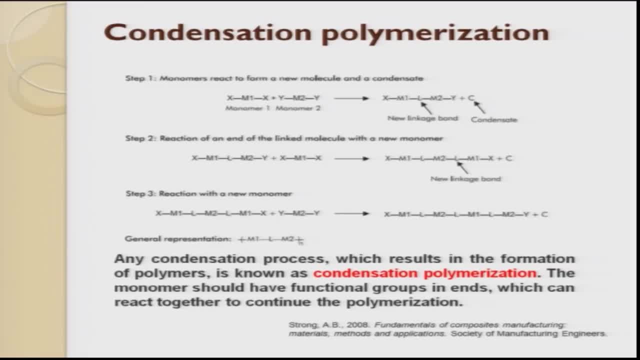 the reaction of an end of the link molecule with a new monomer happens and this reaction with the new monomer keeps continuing and finally it forms a chain. any condensation process which results in the formation of a polymer is called as condensation polymer. 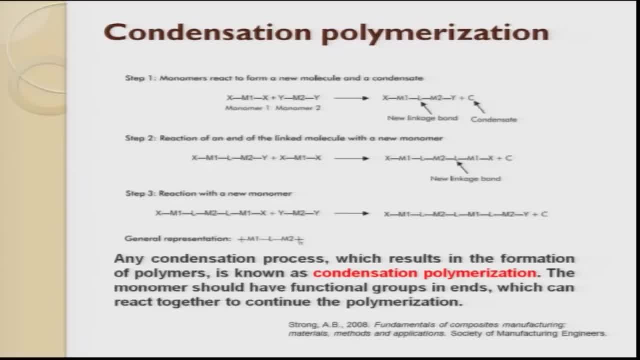 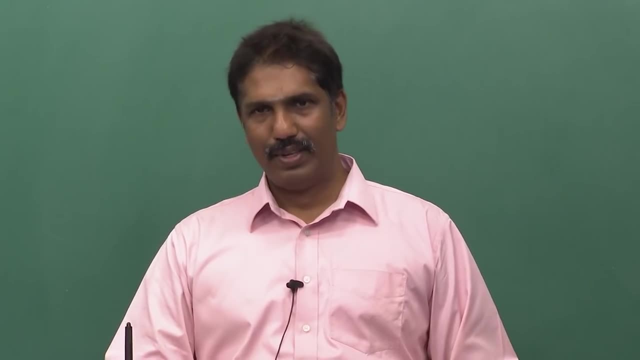 The monomer should have functional groups in the ends which can react together to continue, continue for polymerization. So these are the two predominant mechanism of polymerization happening such that a mer is converted into a polymer. So in, so now the polymer is ready. 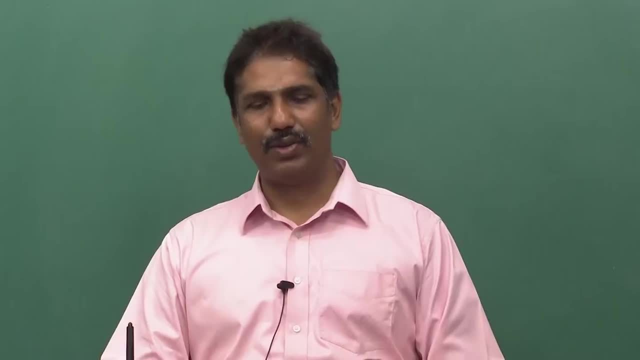 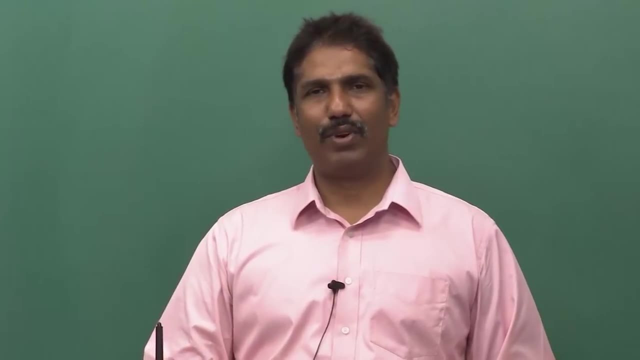 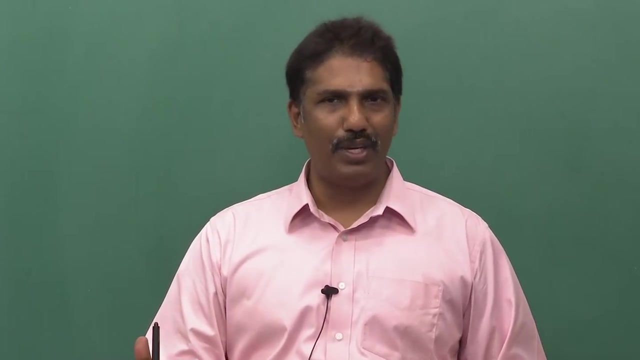 So we will try to add reinforcement to make it into a composite. So I would like to conclude today's lecture. In today's lecture, what we saw was: we saw what is a composite, what are the applications of composite, what are the properties of composites. and we saw different. 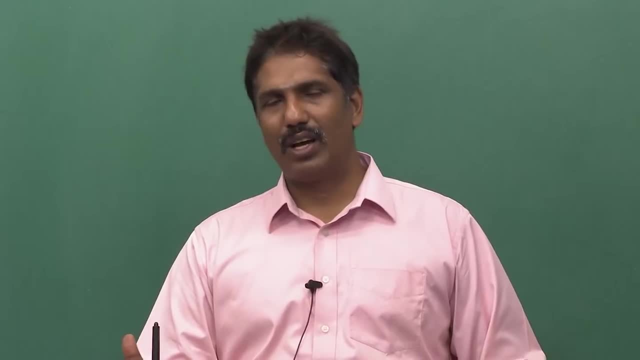 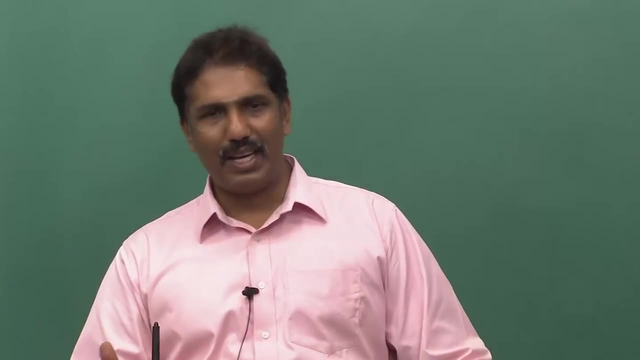 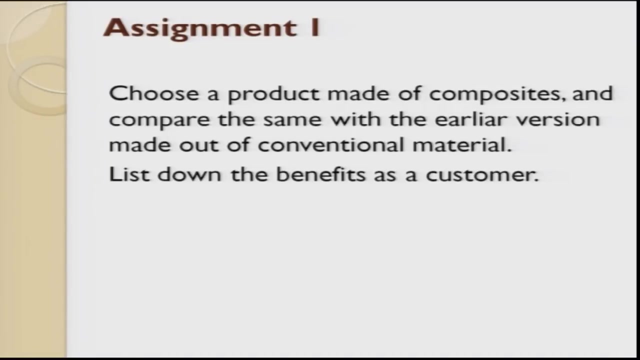 polymerization mechanisms such that how a mer is converted into polymer. We saw only the major mechanisms. So as an assignment today we will try to have, we will have first assignment based on this lecture. So the first question is: you use internet as your source, search for a product which